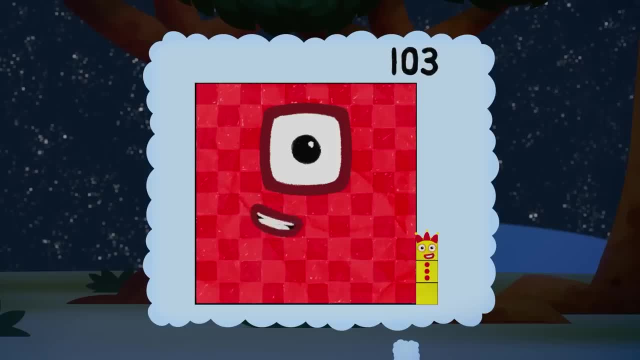 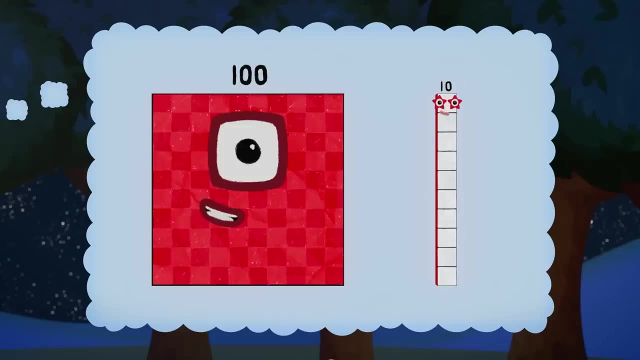 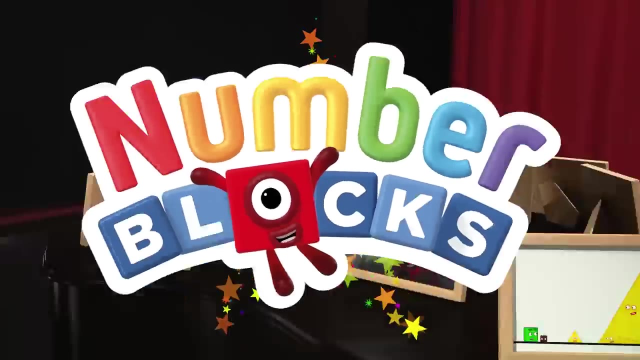 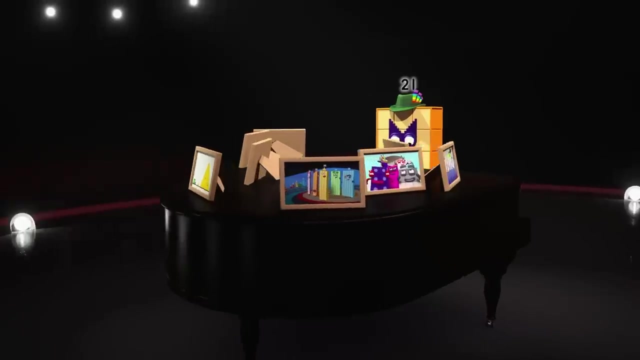 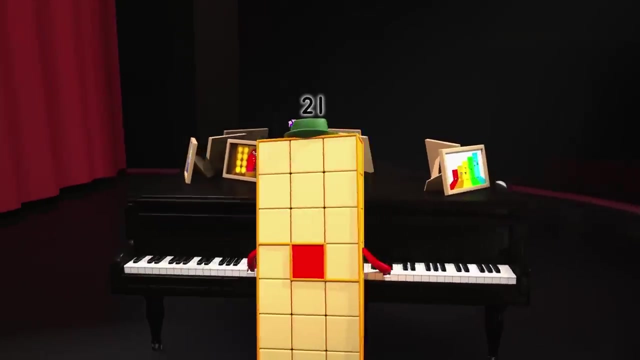 102, 103.. Oh, we can add 10's, 110,, 120,, 130.. We've had such a lot of big adventures. We've had such a lot of big adventures And everyone has played their part. 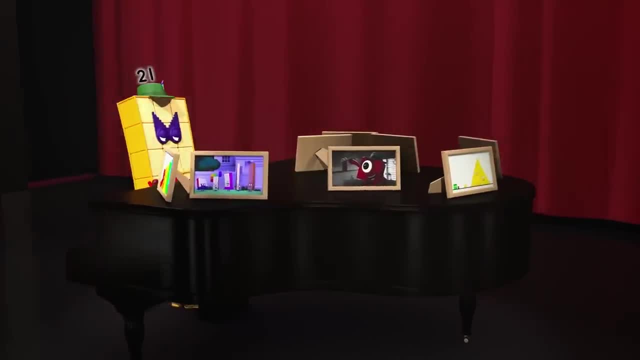 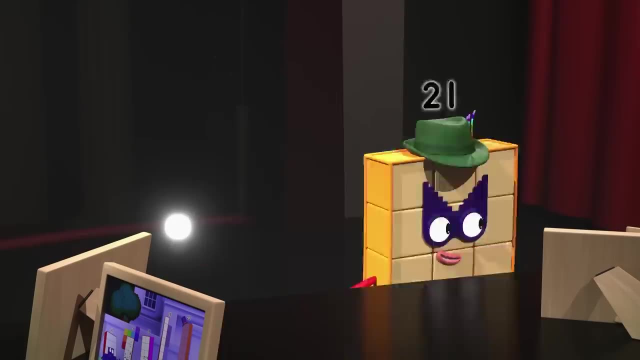 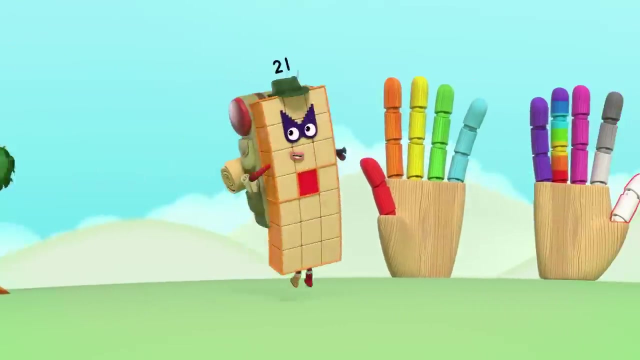 Now it's time to take your turn. You'll be happy to learn. This is not the end, it's the start. There's so much more to explore. You can take a look now. we've opened the door. When we ran out of fingers, we counted our toes. How high can we go to? 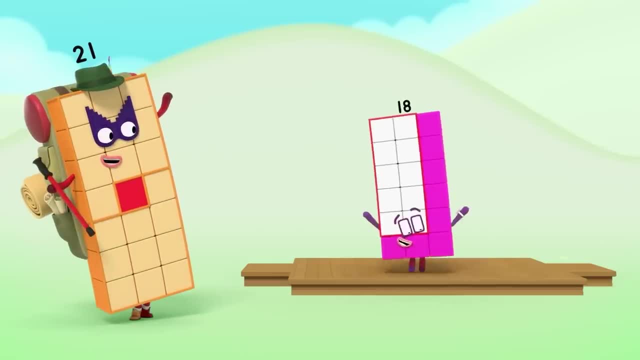 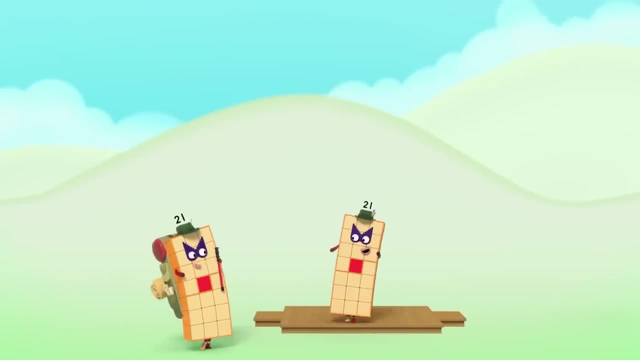 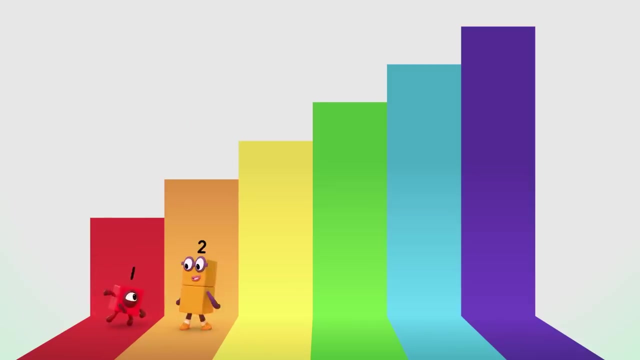 Who knows? If you start with a number for fun, You can make it bigger. if you just add one, You can do it yourself. now you know how it's done. Take the floor. There's so much more to explore. There's so much more to explore. You can add a clock, as you've done it before. When we all get together, we make a new friend, There's gonna be magic, no end. 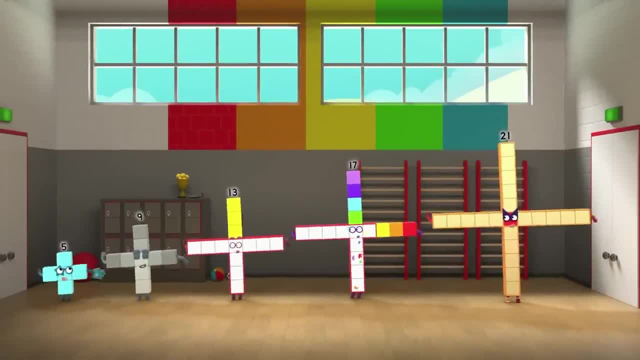 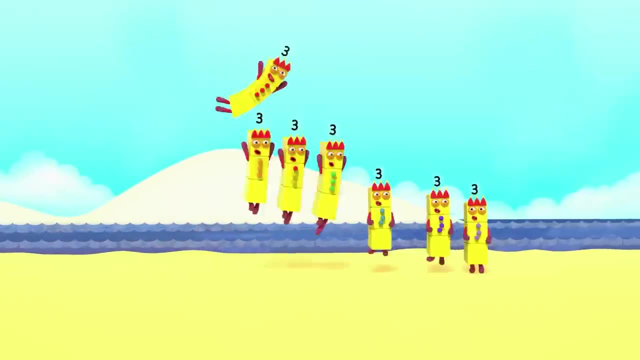 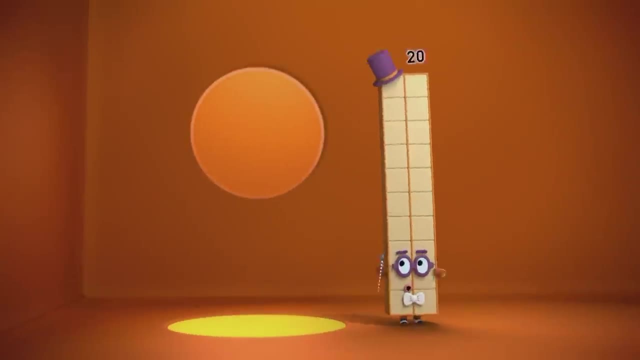 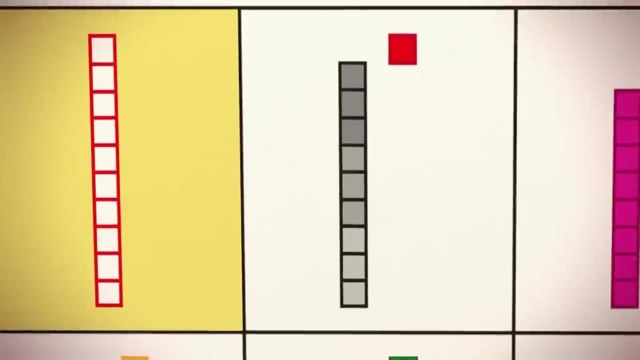 It's a plus. you've got us on your side. Soon you'll find, your fortunes will be multiplied. You've got all of the tools it took to you to decide what they're for. There's so much more to explore. Ha ha ha. Tip top, Two high up buttons to tap, And I know the pair to do it. If 10 can make 9 and 1, then I can make. 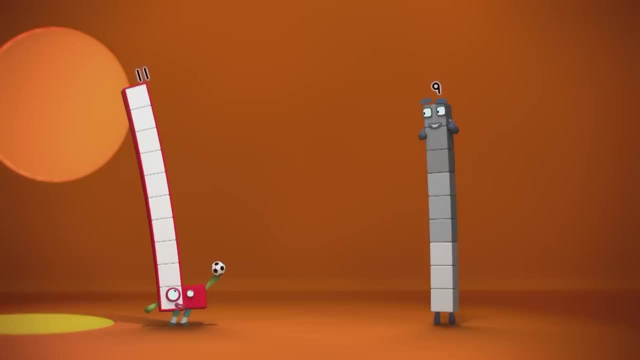 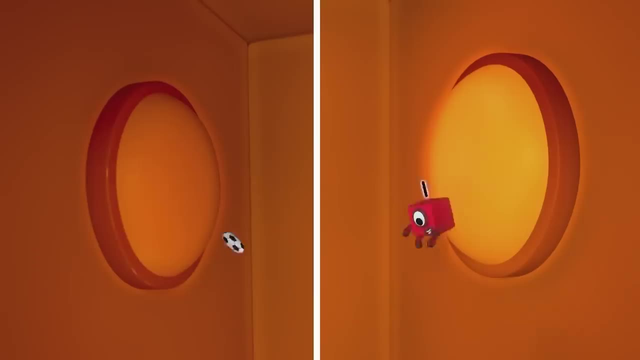 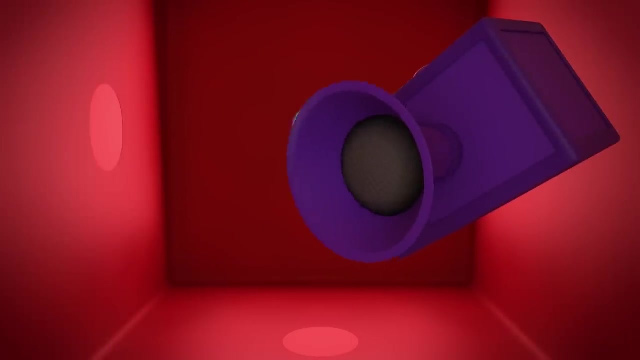 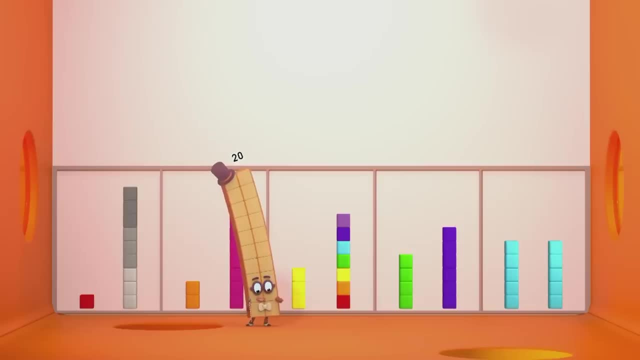 I can, I can. I'm 10 and 10, so my 20 friends are the same as 10's 10 friends Plus another 10.. 11 and 9 or 1 and 19.. 12 and 8 or. 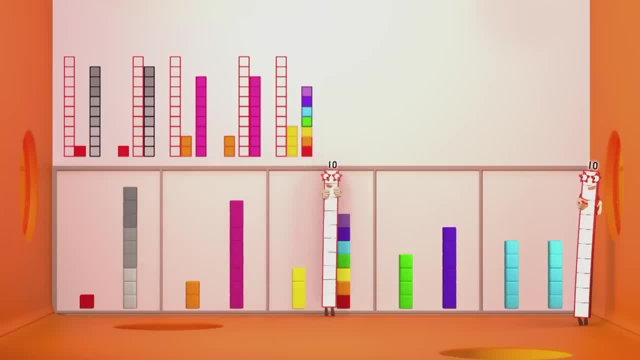 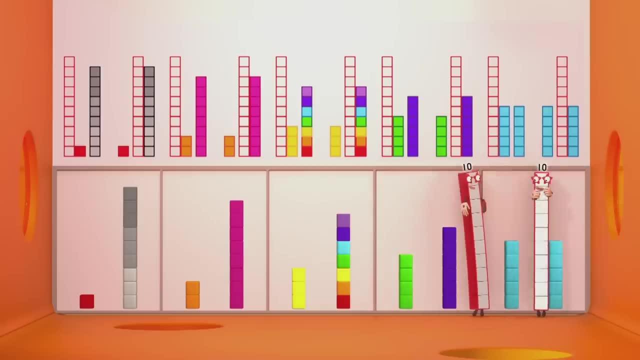 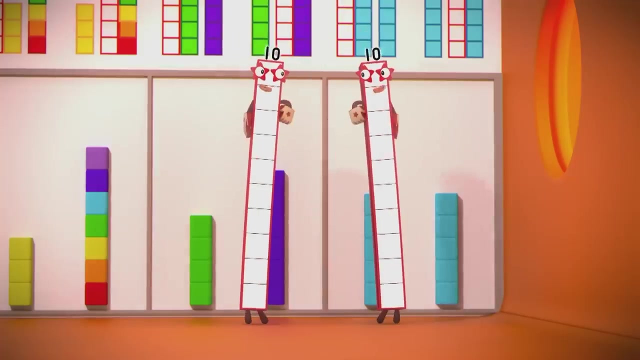 Or two and eighteen, Thirteen and seven Or three and seventeen, Fourteen and six Or four and sixteen And fifteen and five, Either way round. If I'm ten more than ten, I can also make Two tens Blast off. 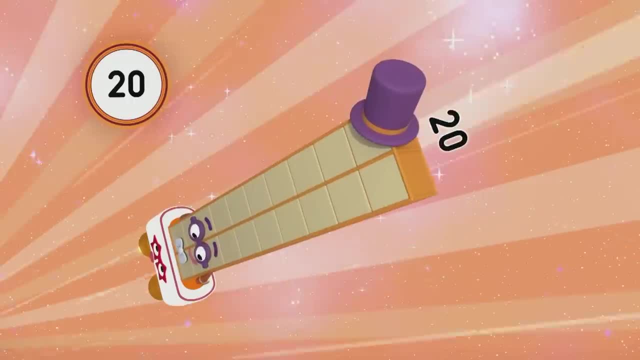 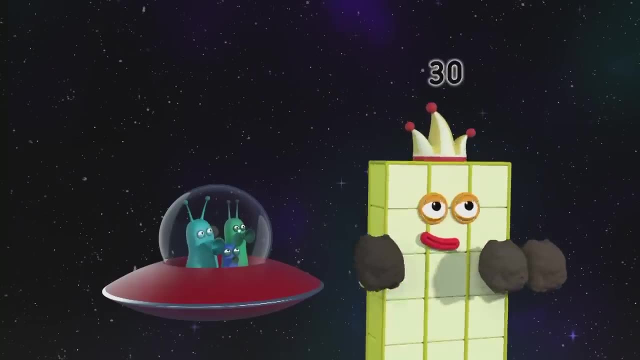 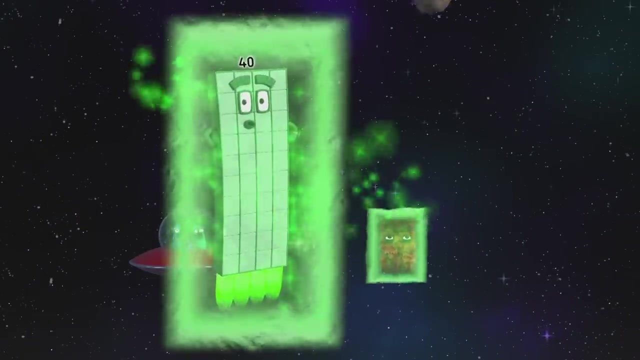 Woohoo, Thirty juggles asteroids. You ain't seen nothing yet. The greatest show in space Forty is a rectangle with an oblong pit. It's a galactic oblong Three. They know what their zero's for. 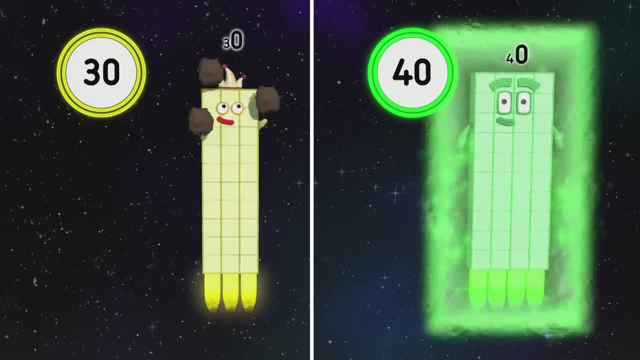 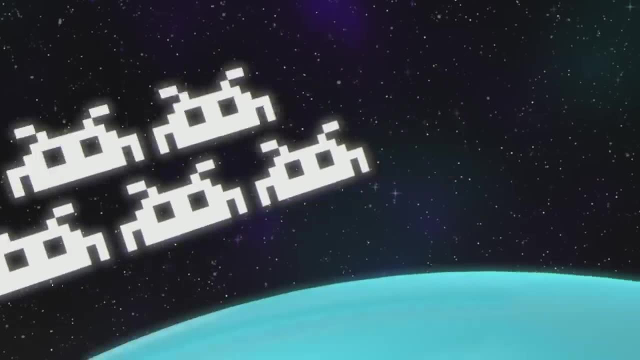 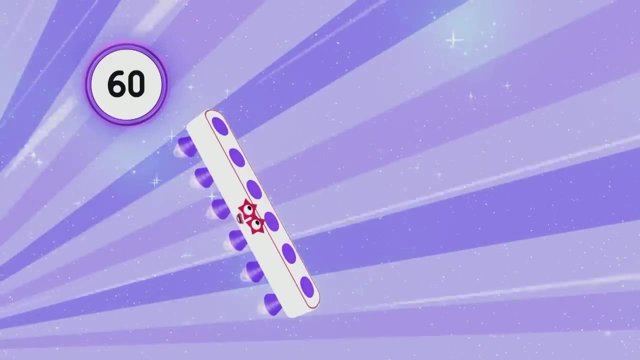 Three tens, four tens And nothing more. Heroes with zero's. Fifty is a superstar Who works the satellites Interstellar overdrive. Yay. Sixty is a super gamer: She can light the lights Galactic game over. Yay. 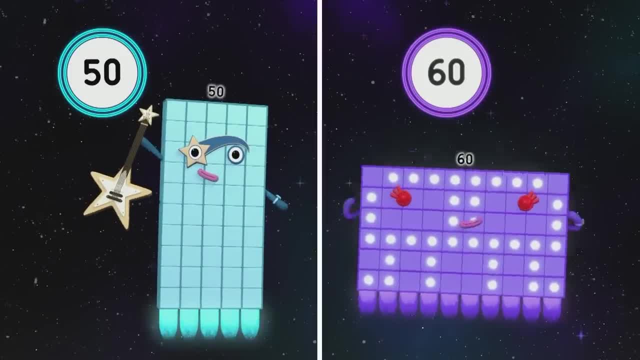 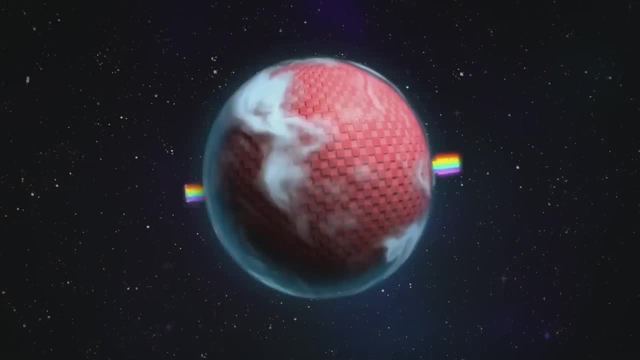 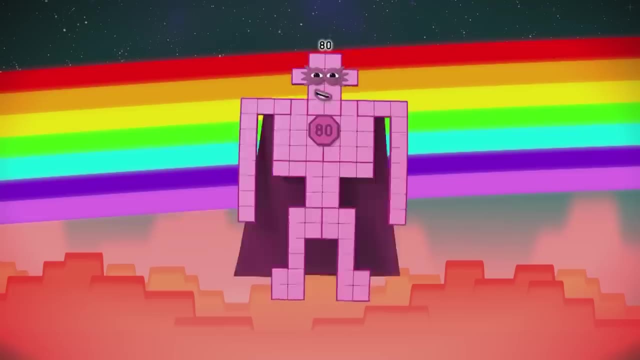 Five tens six tens. Heroes with zero's. Seventy has luck times ten, Launching from the dock Space rainbow. Oh Eighty needs no luck at all, He's super rock the block, Dinocto block, Robocto block. 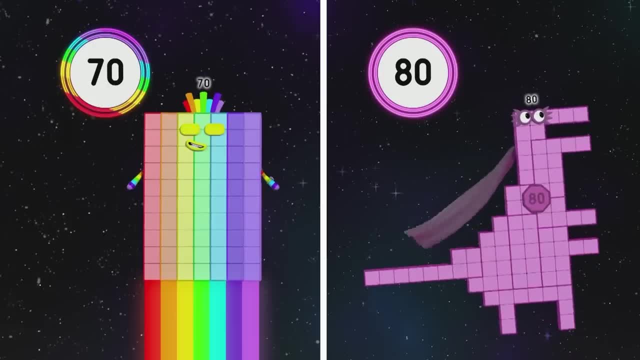 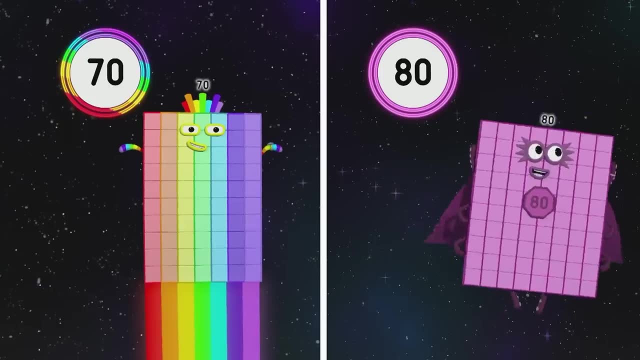 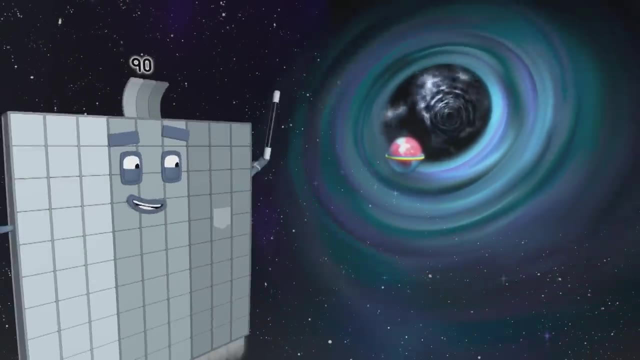 Dinocto block Roblox. They know what their zero's for: Seven, tens, eight tens And nothing more. Heroes with zero's Ninety knows a trick or two. He will heed the call Abracadabra. And now let's meet one hundred. 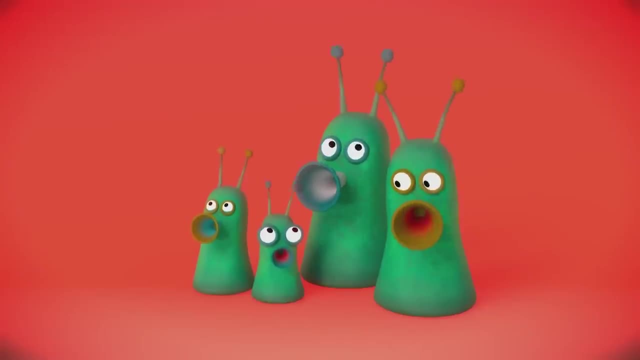 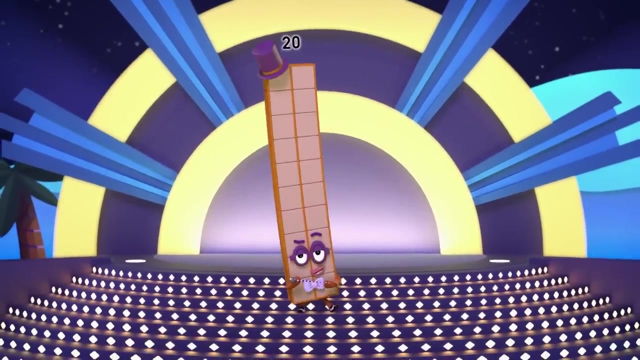 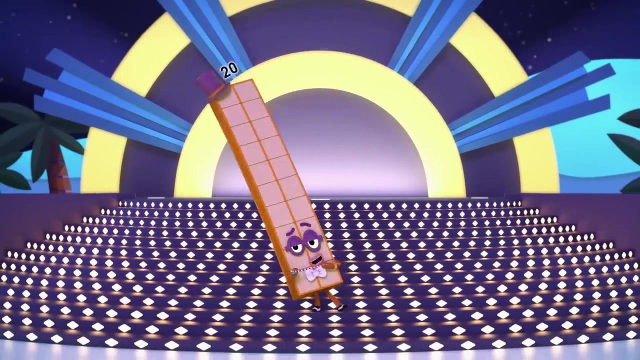 The greatest of them all, Three Hero with two zero's Ten, twenty, and I love to dance With plenty of moves to my name: I'm tall and I'm slender, I'm graceful and gender. I sway as I do the furndangle. 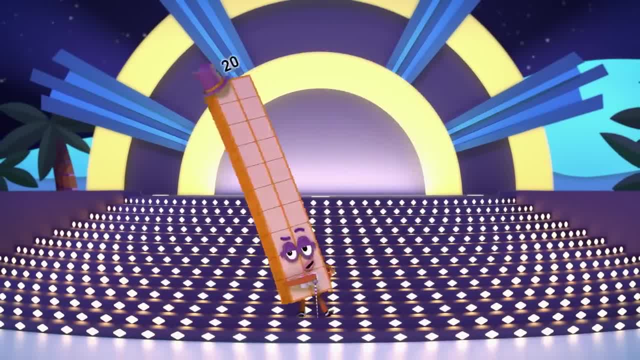 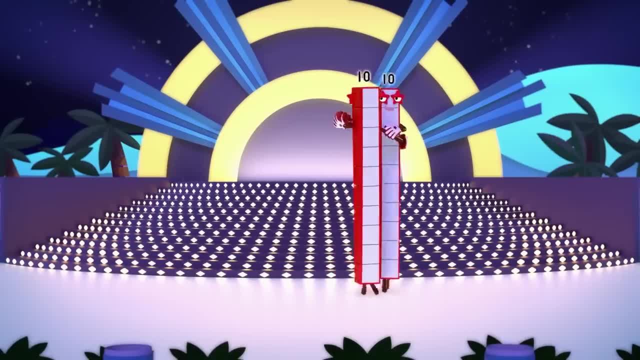 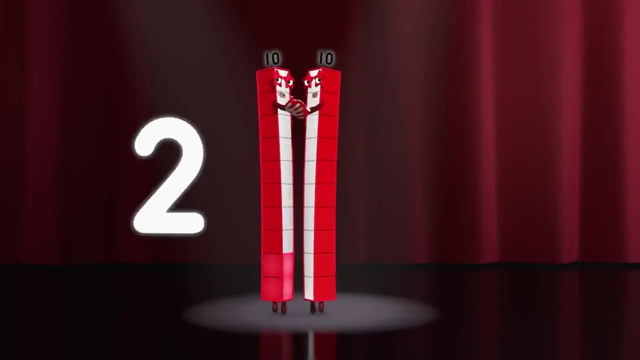 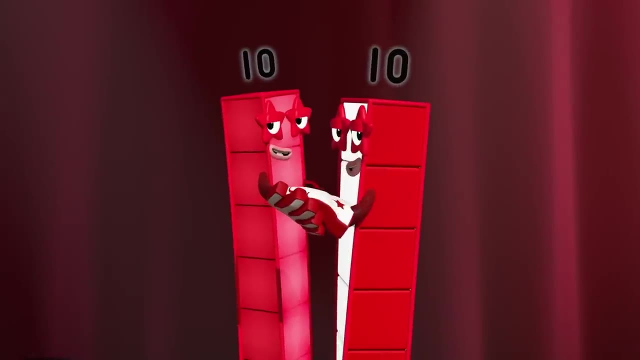 Two tens, nothing more. as I take to the floor And dance to the two ten tangles- Four, Five, Four, Five, Six, One, two, three, four, five, six, seven, eight, nine, ten, Drop to the floor and go round again. 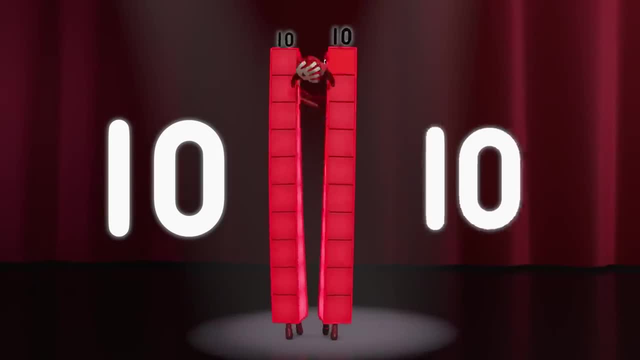 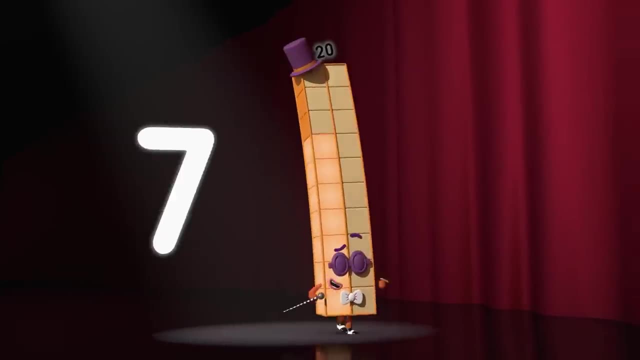 One, two, three, four, five, six, seven, eight, nine, ten. Two friends, two tens make twenty. One, two, three, four, five, six, seven, eight, nine, ten, Halfway to twenty. go round again. 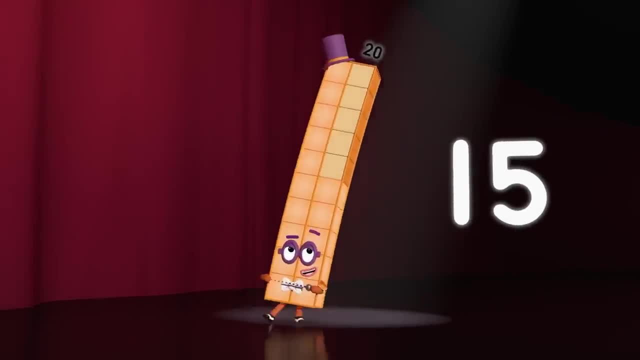 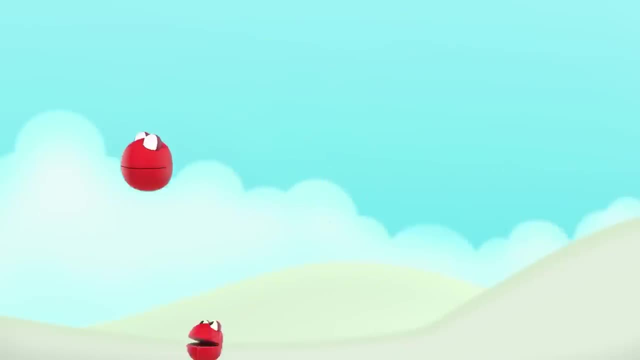 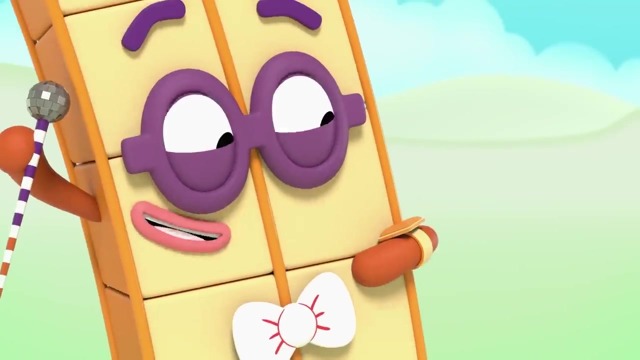 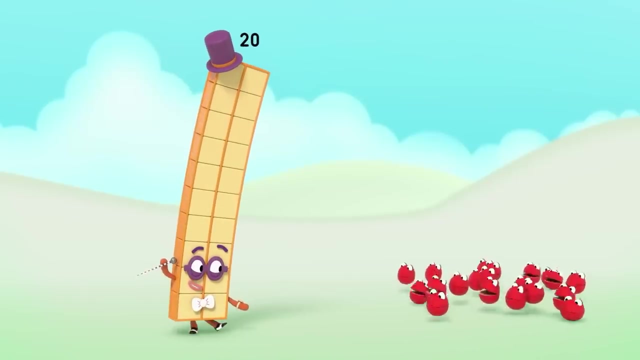 Eleven, twelve, thirteen, fourteen, fifteen, Then sixteen, seventeen, eighteen, nineteen, twenty. Can you count to twenty? I can count to twenty. We can count to twenty. Let's all count to twenty. I can count to twenty. lighting up my blocks. 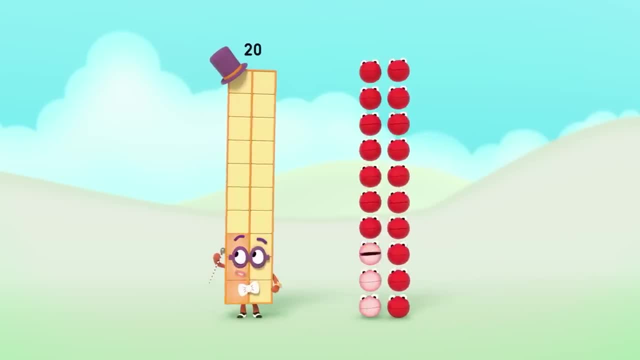 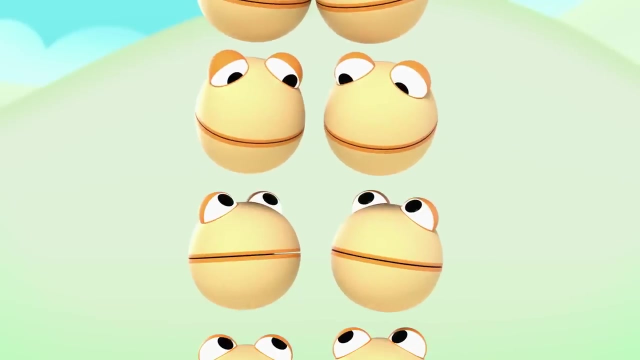 We can count to twenty like a bunch of bouncy rocks: One, two, three, four, five, six, seven, eight, nine, ten, Eleven, twelve, thirteen, fourteen, fifteen, Sixteen, seventeen, eighteen, nineteen, twenty. Can you count to twenty? Tapping on your nose? 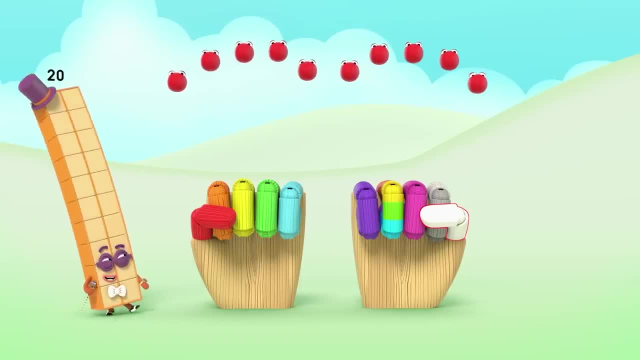 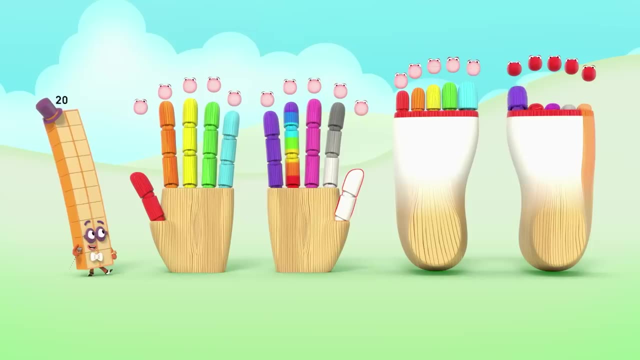 We can count to twenty on our fingers and our toes: One, two, three, four, five, six, seven, eight, nine, ten, Eleven, twelve, thirteen, fourteen, fifteen, Sixteen, seventeen, eighteen, nineteen, twenty. Who can count to twenty? 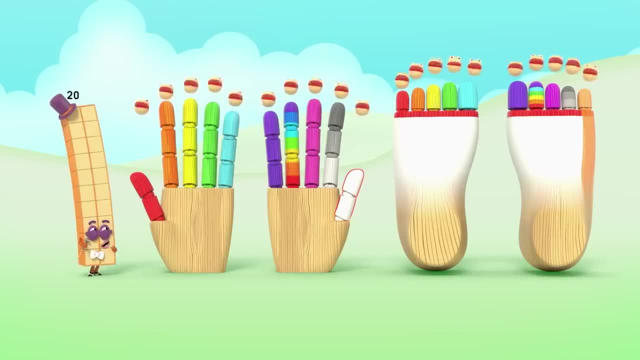 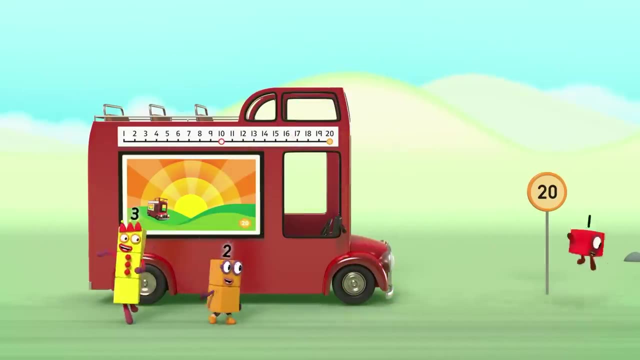 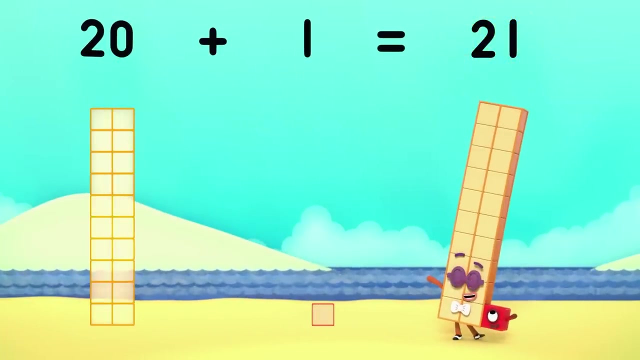 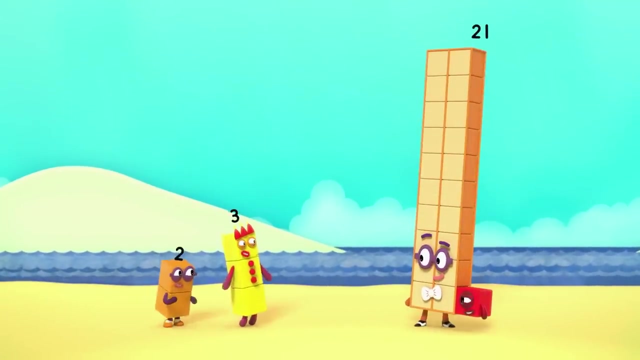 You can count to twenty. We can count to twenty. Let's all count to twenty. Let's explore: Twenty plus one equals twenty-one. I'm twenty-one, I'm twenty and one. You're twenty-one. You've got two faces. Sometimes it's easier to think of bigger numbers. 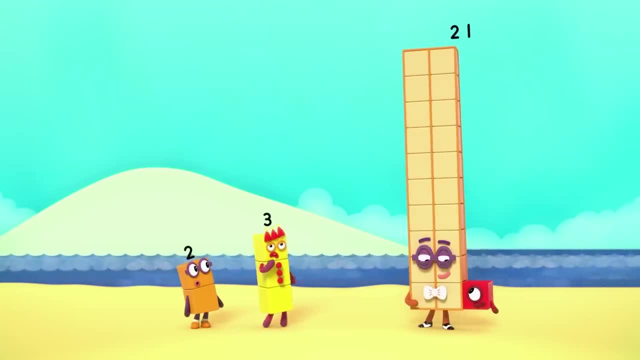 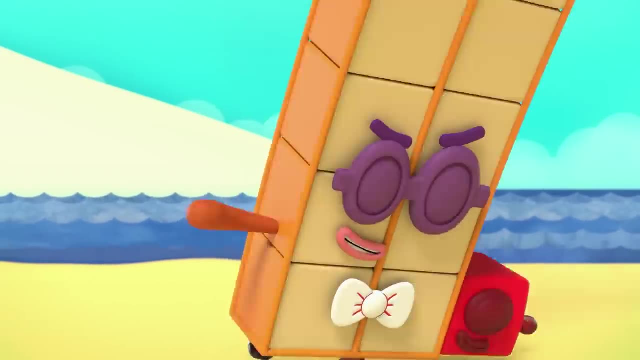 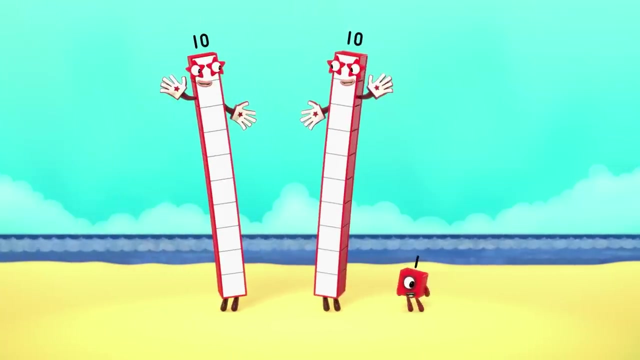 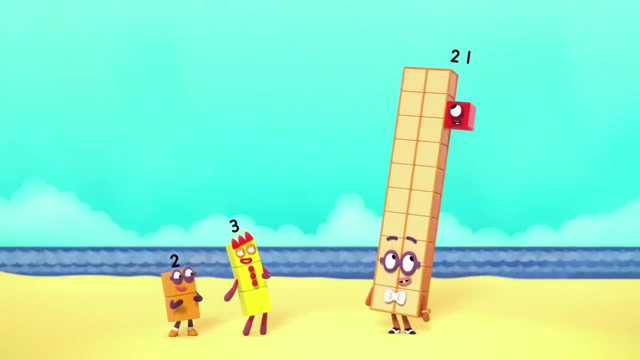 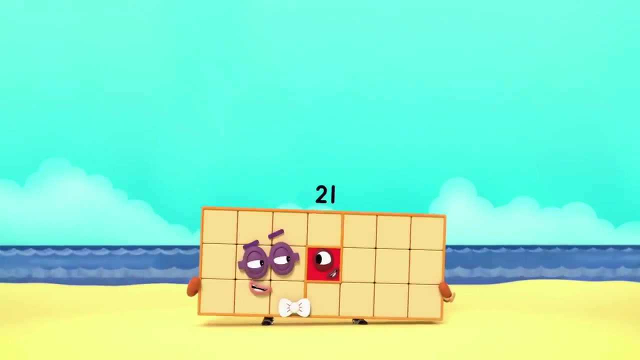 Two numbers together: Twenty-one, Twenty and one. Oh, I see, I wonder who else I can be. That's me. twenty-one. I'm two tens and one-one. Two blocks wide leaves an odd block on top. I'm an odd number And if I do this, I can be. 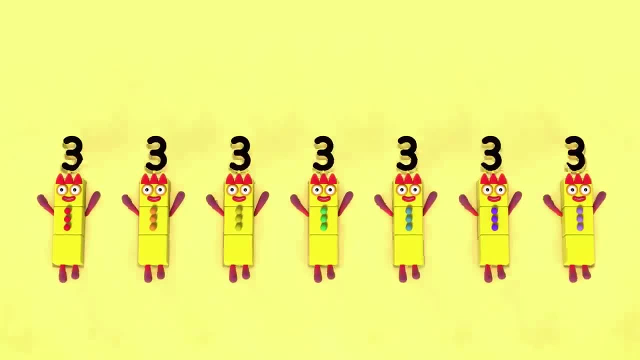 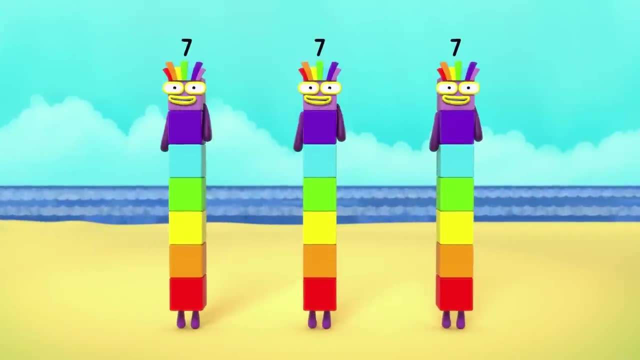 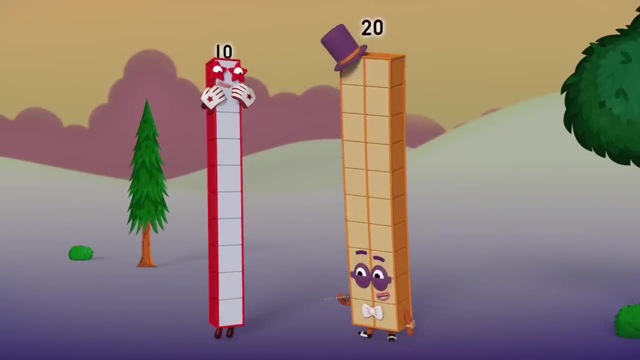 Seven, threes, What? I'm also three sevens, Which means I'm also Three sevens. Look a treasure chest. You know Three, there's someone you should meet. Huh Who? Well, I'm one ten And I'm twenty. 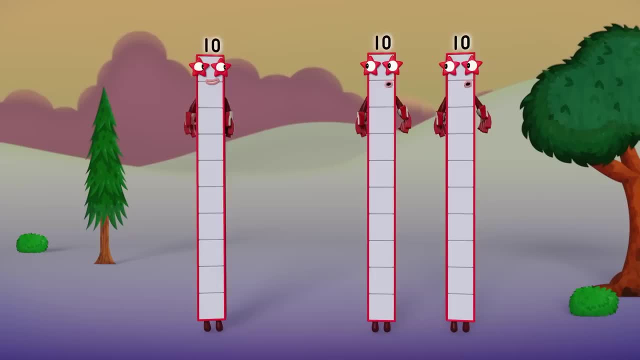 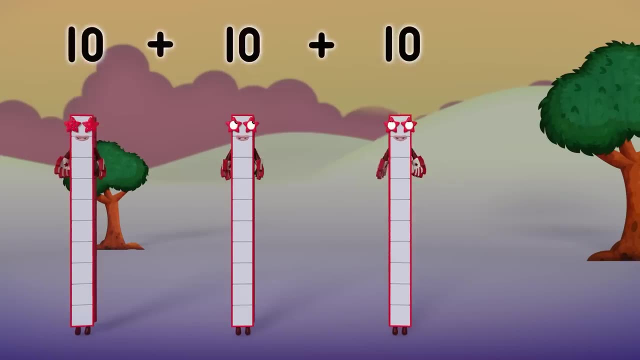 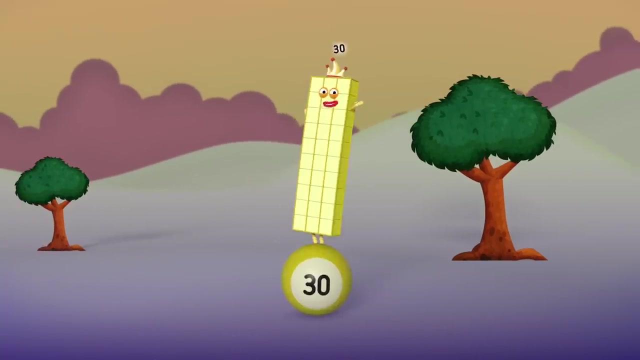 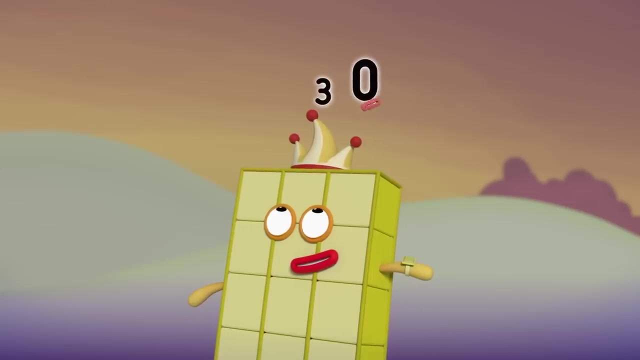 I'm Two tens. Put us together, and what have you got? Three tens. Ten plus ten plus ten equals thirty. I am thirty, the big entertainer. This three stands for three tens, And nothing more. Oh, If you'd like to see more, then come to the. 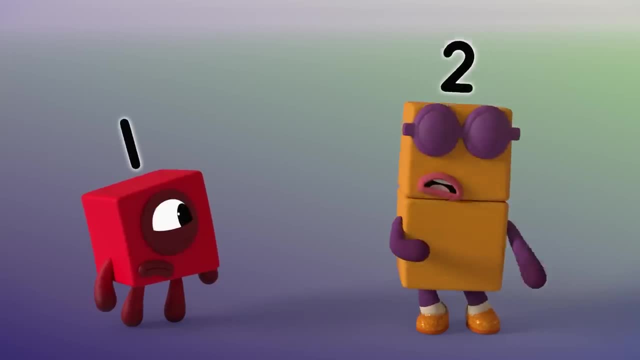 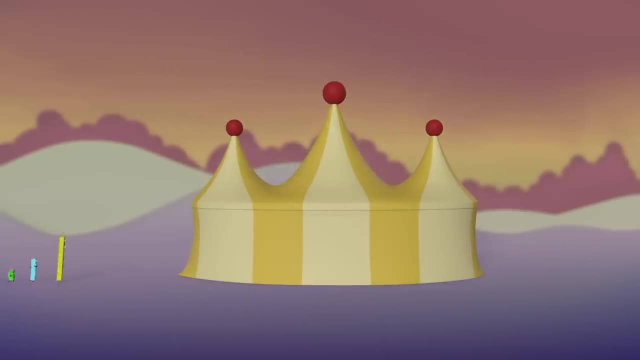 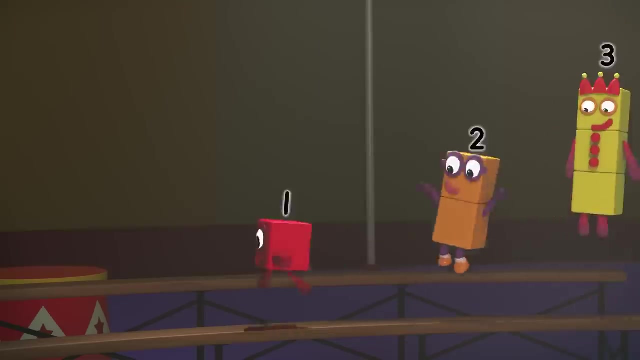 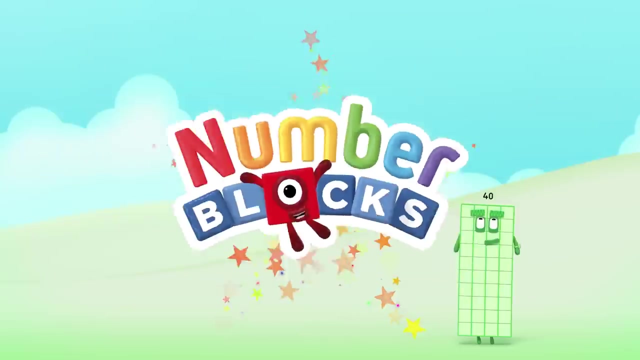 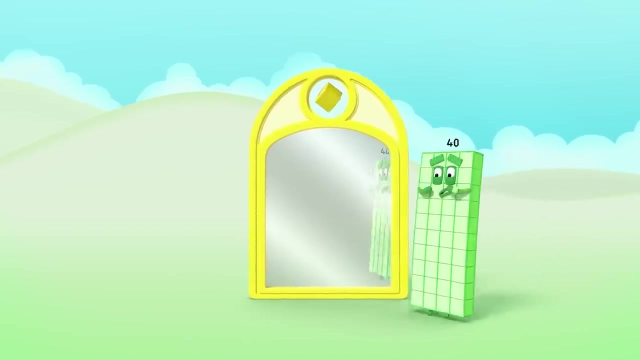 Circus, What circus. I like to keep it Under my Hat. Welcome to the big, big, big Top. I love rectangles. Would you like to meet my pet rectangle? Oblongy, Oblongy, Oblongy. 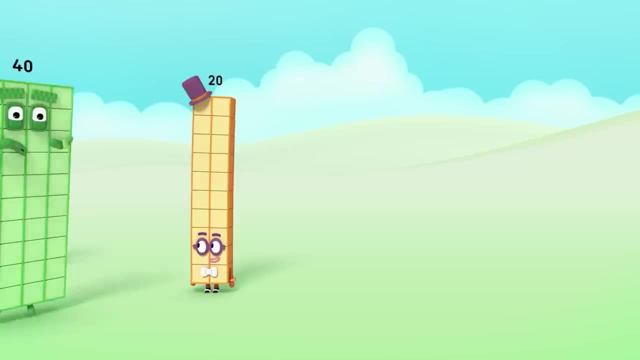 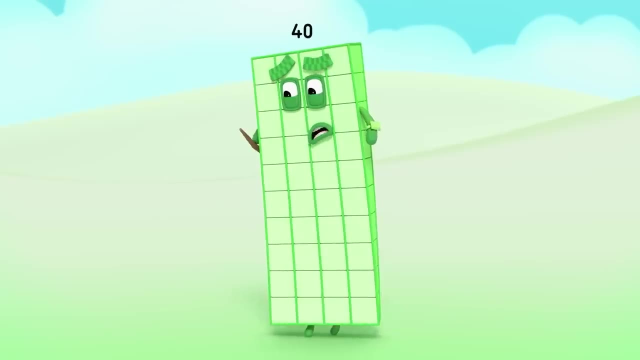 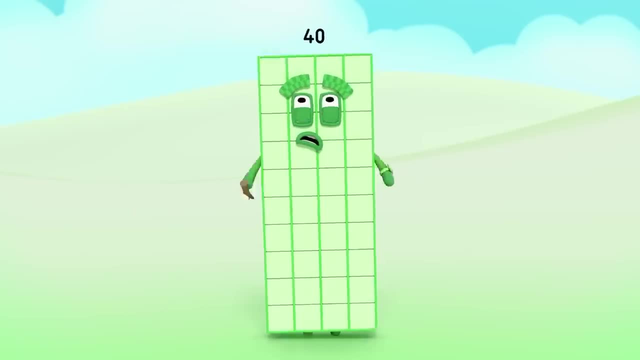 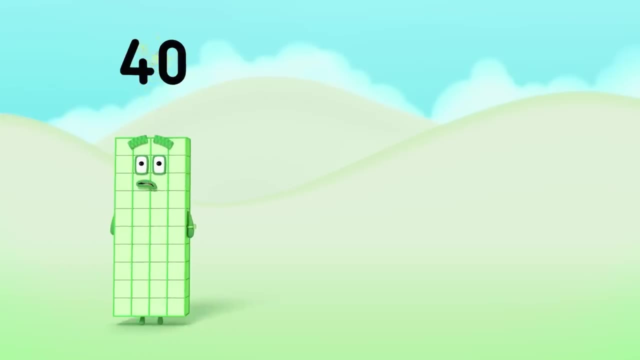 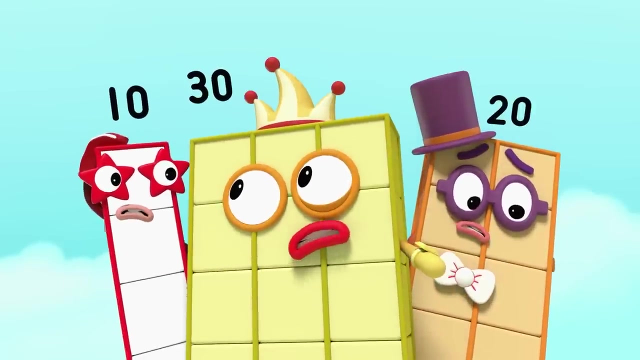 Left or right. I can't go both ways, But we can. Oh no, Not you. two Forty equals twenty Plus twenty Two. lots of 20 feathers. It's tickling time, Tickle-tickle. Hey, Come back here. 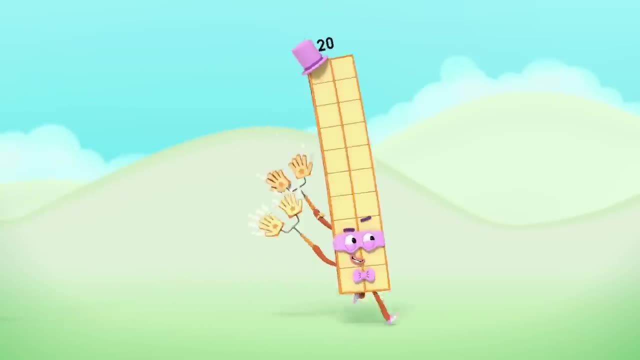 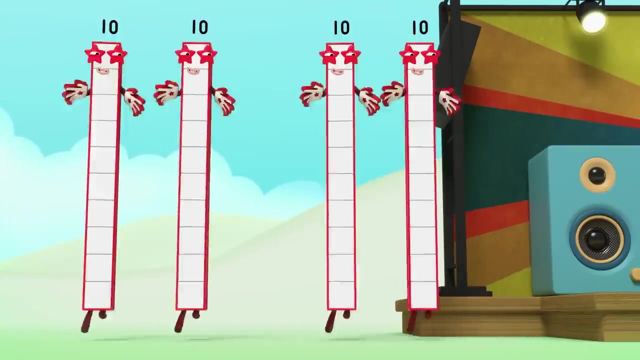 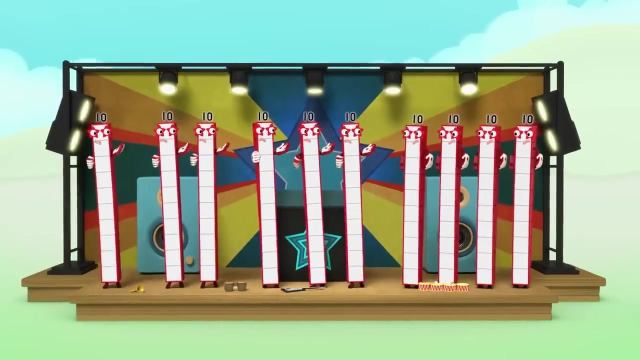 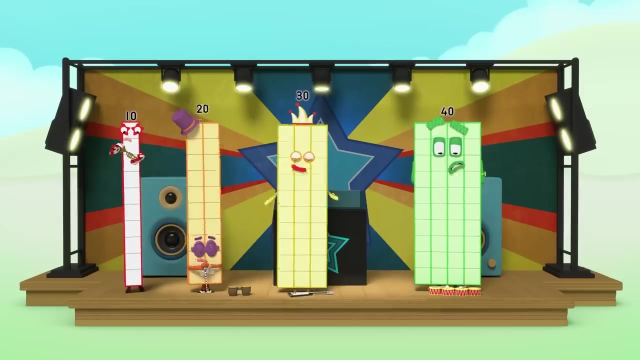 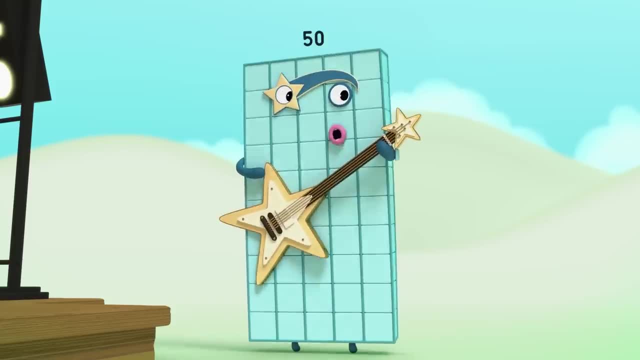 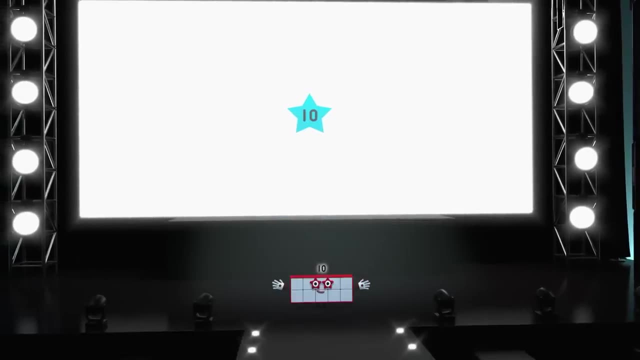 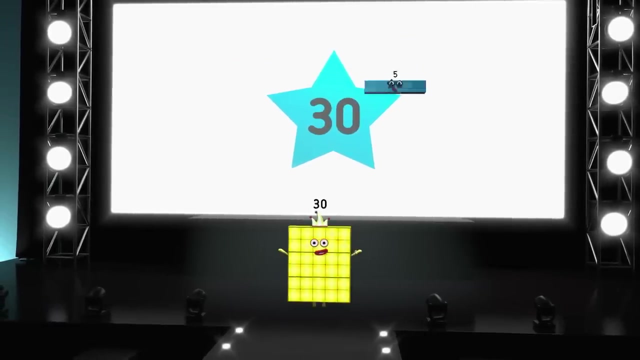 Whoa, Woo-hoo. Hey, who turned everything up to 10? Five, 10. 15., 20., 25., 30., 35., 40., 45. And 50! Let's rock. 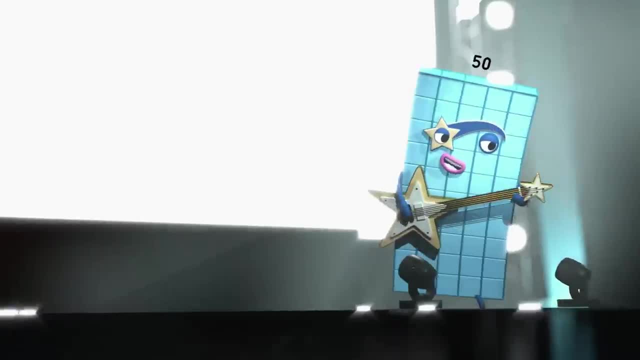 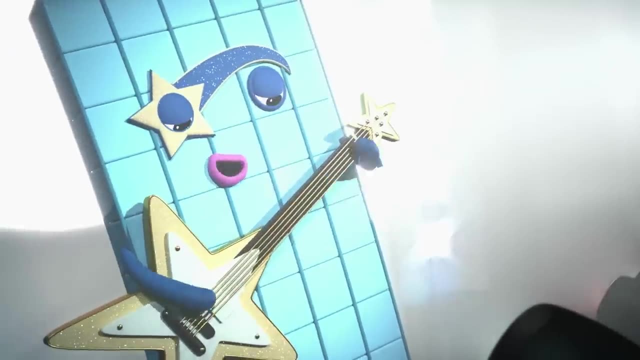 My name is 50.. I'm a rock and roll super star. I'm all the rage when I take the stage with my shining gold guitar, And so you don't forget my name. I play this counting game in 5, 5,, 10,, 15,, 20,, 25,, 30,. 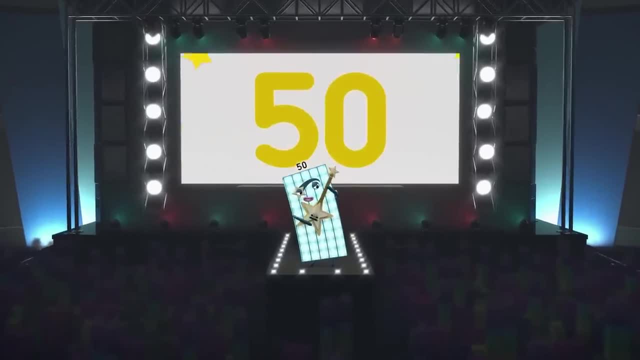 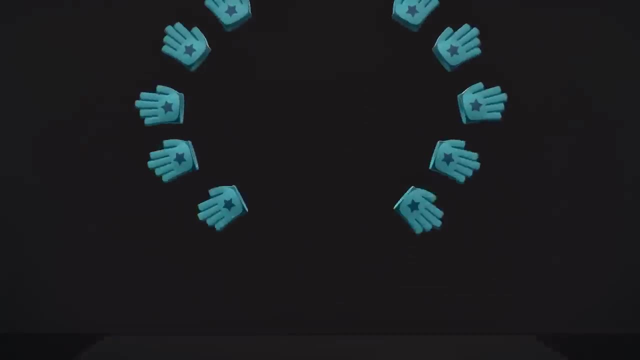 35,, 40,, 45, and 50.. I'm 50.. Huh, 10 hands, 10 big hands flying through the air. Count the fingers super quick, with a little bit of flair, Five fingers on each hand. 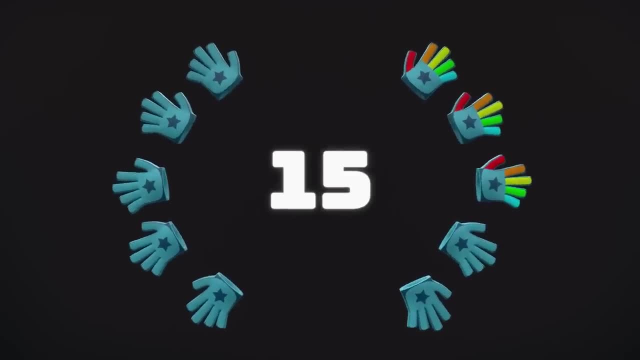 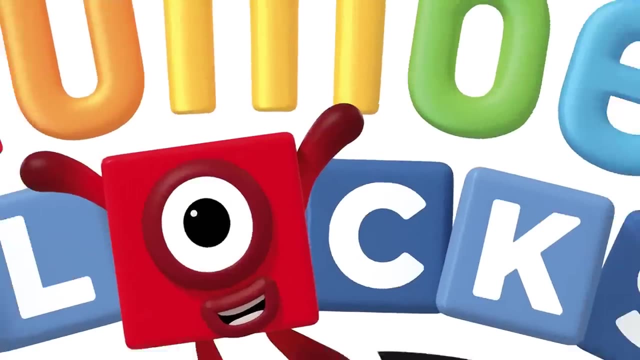 High five: 5,, 10,, 15,, 20,, 25,, 30,, 35,, 40,, 45, and 50.. 50 fingers, I'm six, 10s Or 10, sixes. 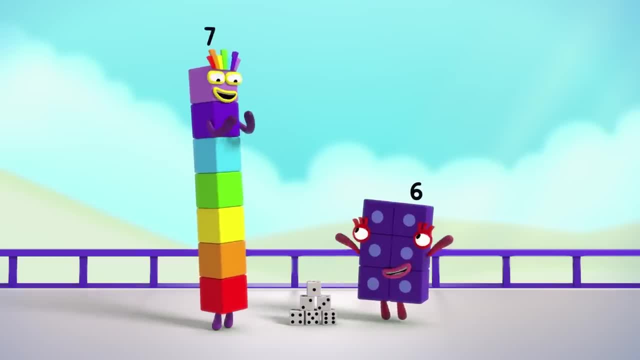 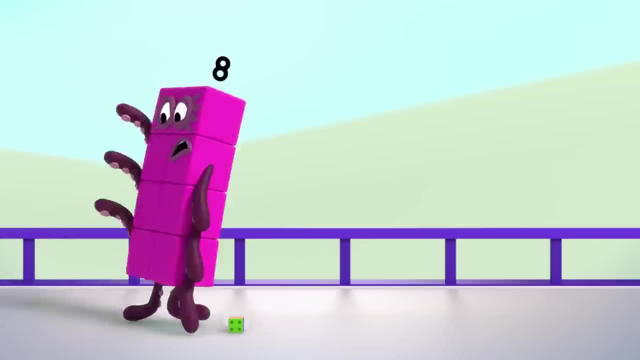 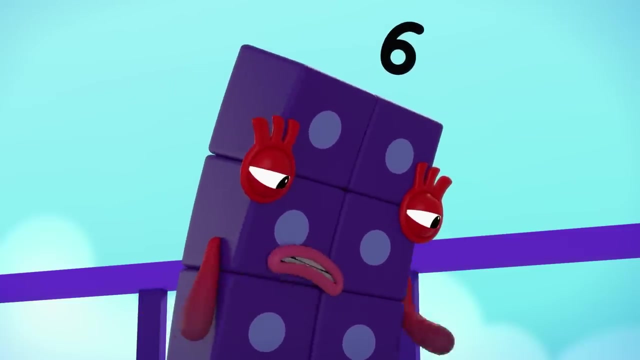 Game on: Yeah, Hey, Huh, Huh, Huh, Huh. Come on nine, We can, Oh, Uh-oh, Oh, Oh no, The special game dice. I'm sure you'll see that dice again. 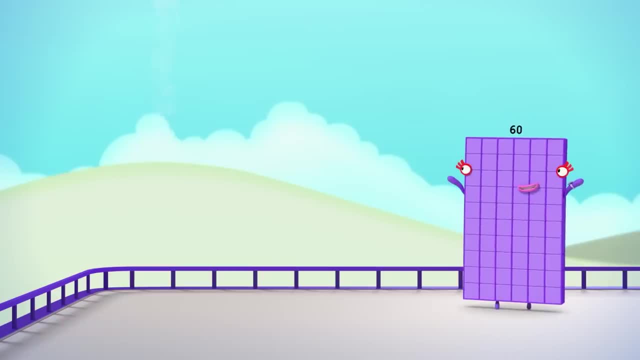 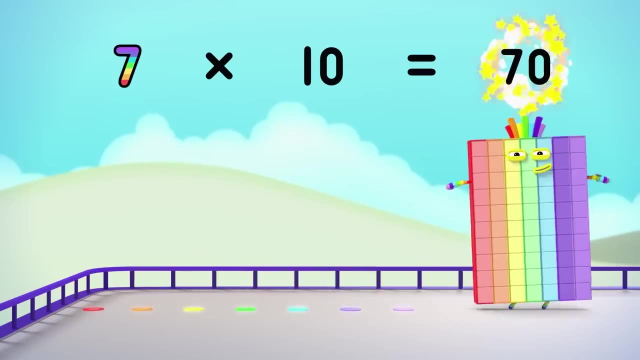 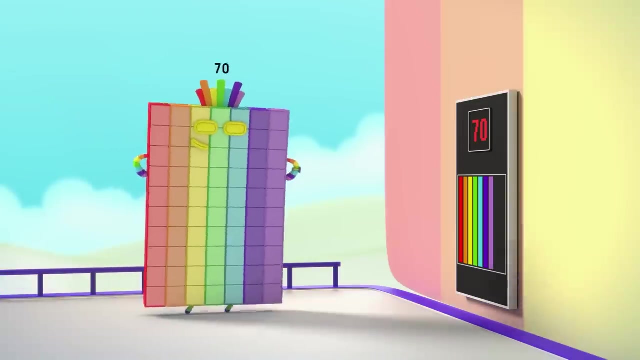 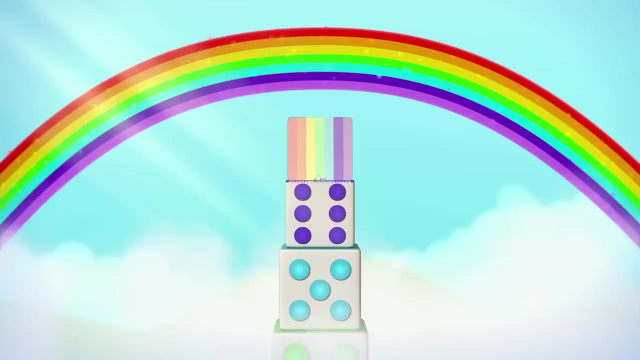 This calls for another 10.. Seven times 10 equals 70.. 70. I am 70. You lucky numbers. As luck would have it, I'm 7 tenths, So I'm also 10 sevenths. 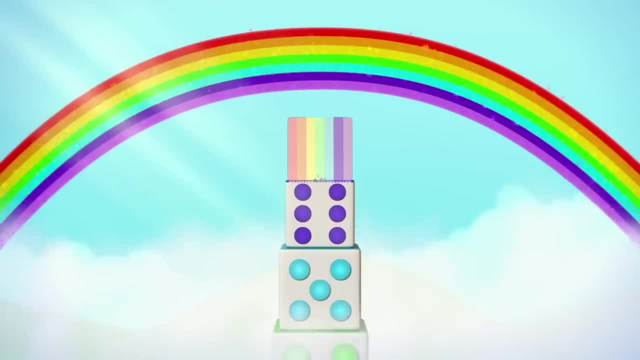 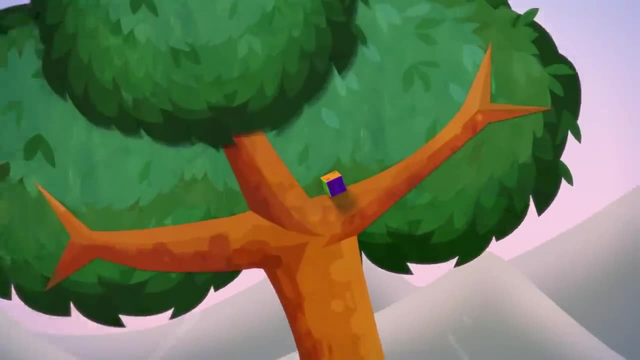 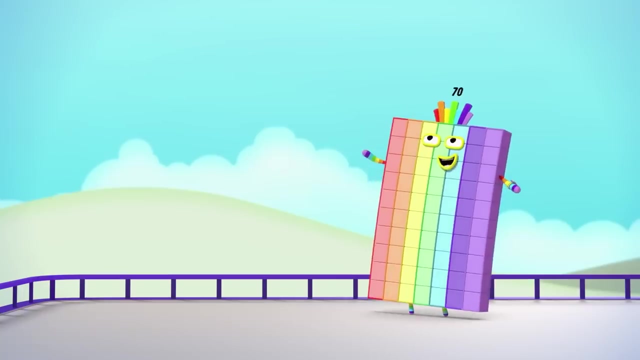 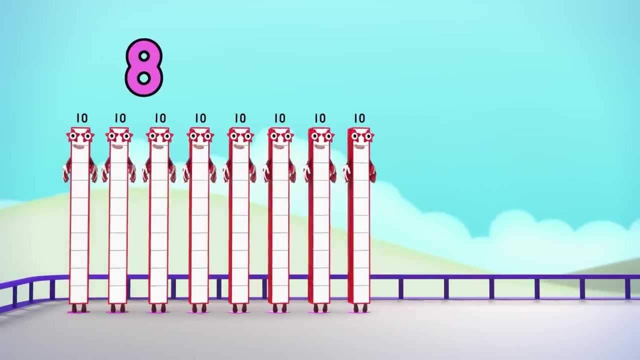 The Rainbow Collection. Ooh, Oh, Oh, Oh. I see it. It's way over there, But how can we get it back again? Luck is in the air tonight. Here comes another 10.. Eight times 10 equals. 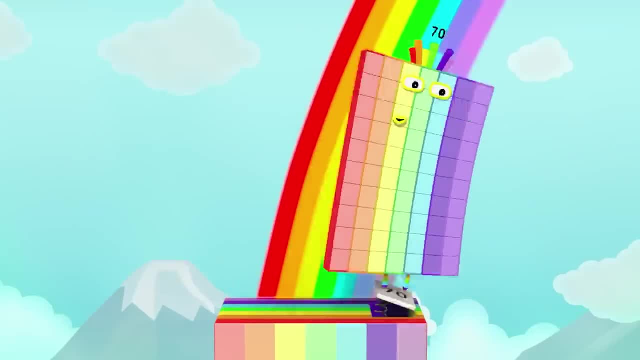 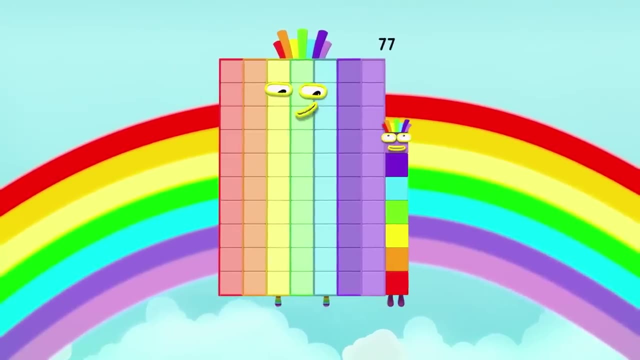 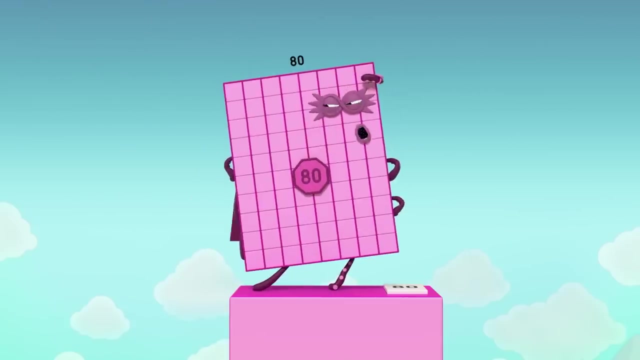 80! Over the rainbow. 71,, 72,, 73,, 74,, 75,, 76,, 77,, 78,, 79,, 80!. Hmm, I don't like the look of those clouds. There's no time to stop. 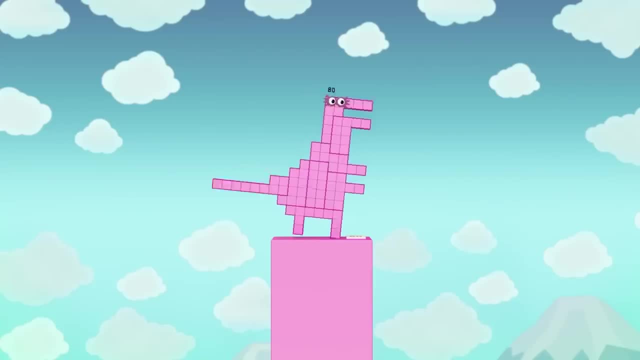 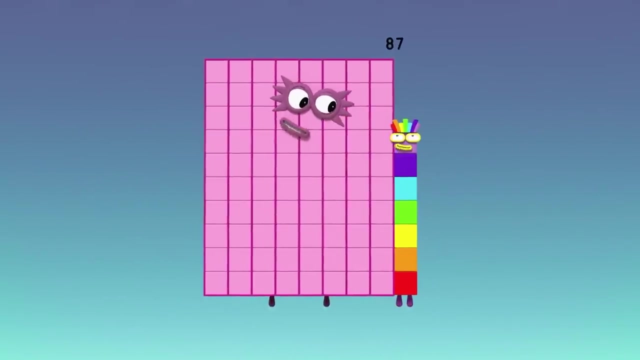 Octoblocks assemble Dinoctoblock, roar, Roar, Oh, Ah-ha, Up, up and away. 81,, 82,, 83,, 84,, 85,, 86,, 87,, 88,, 89,, 90!. 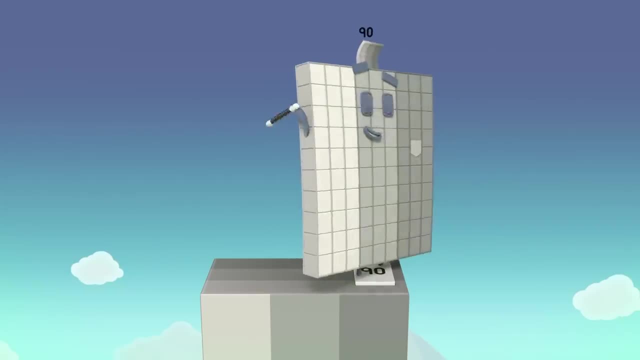 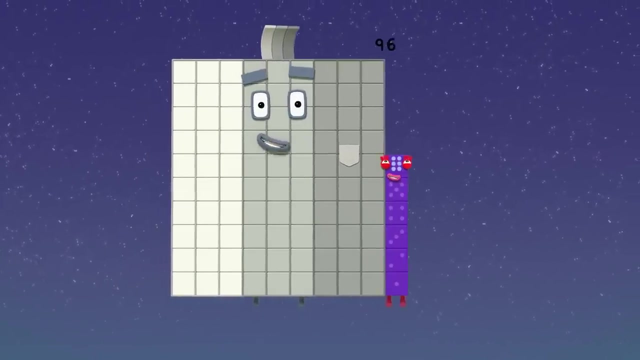 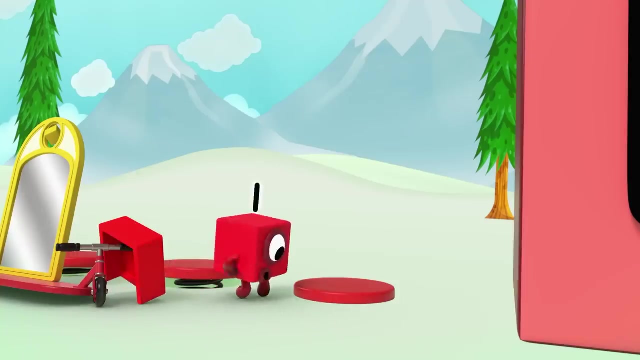 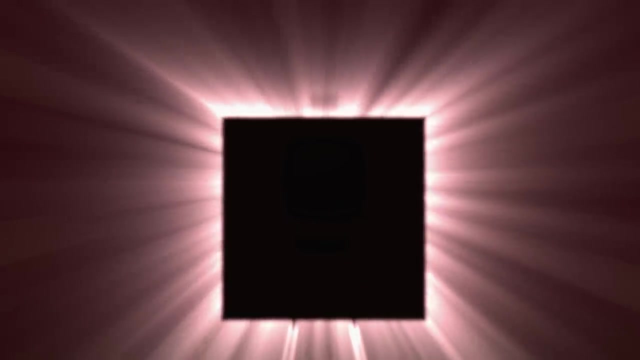 Nearly there, with no time to spare, This should do the trick. 91,, 92,, 93,, 94,, 95,, 96,, 97,, 98,, 99!. And one more is Roar 100.. 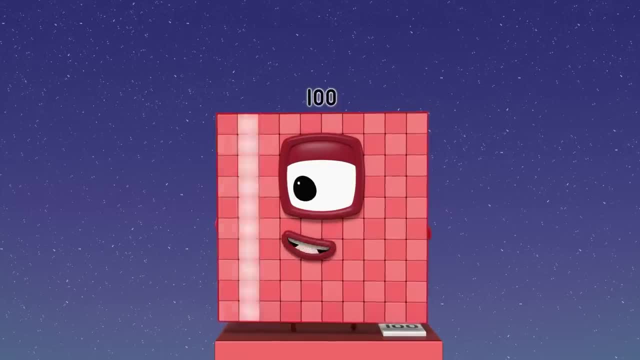 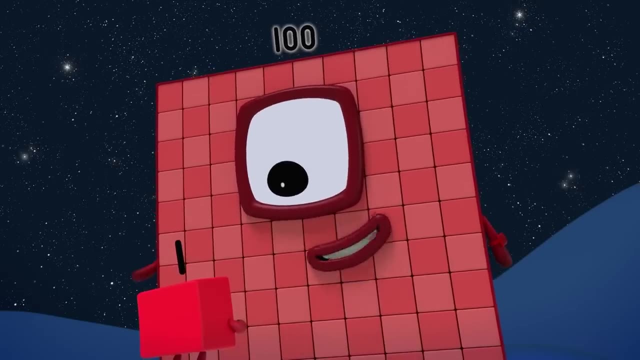 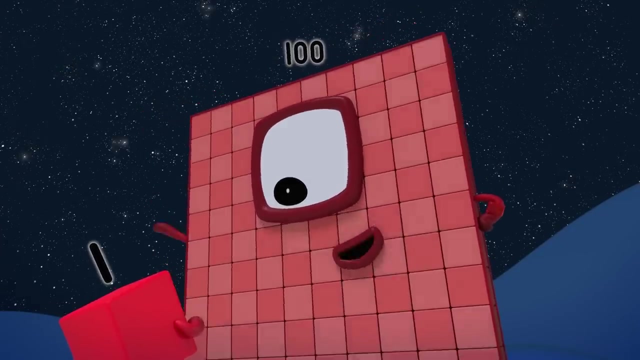 I am 100.. 10, lots of 10.. 100!. Hello one, You're so big. Yes, little one, I'm a big number, But I wouldn't be here at all if it weren't for you, Oh. 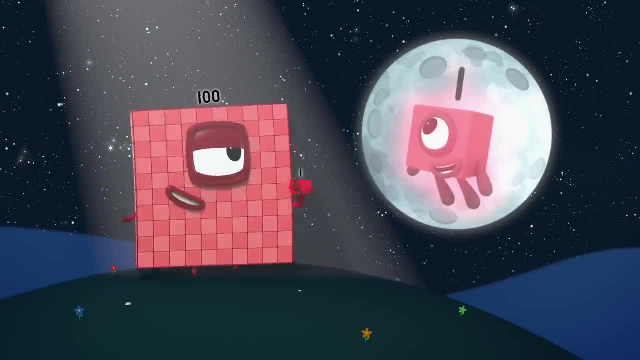 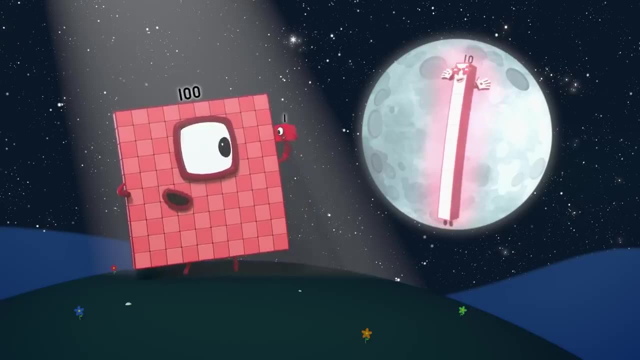 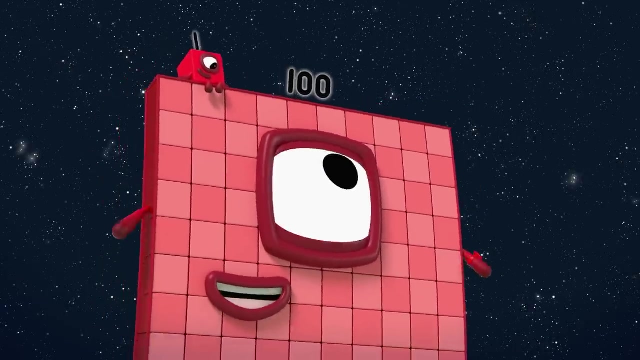 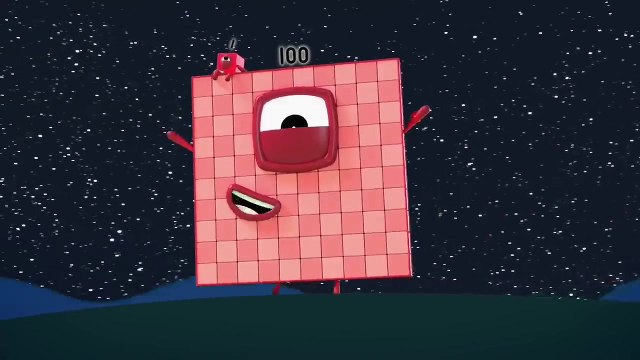 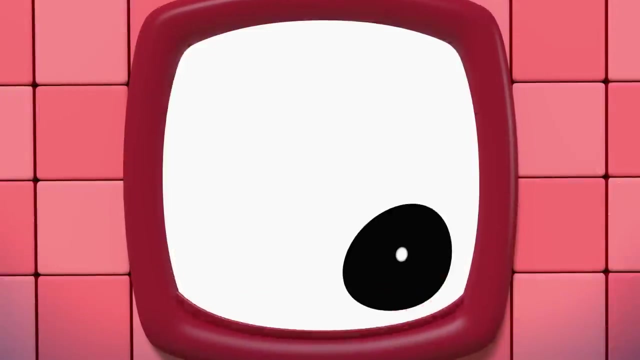 Look how far we've come. Remember when there was only one, Then 10 ones made 110, With a one And a zero. Now we've reached a new place, A place of possibilities, A new friend, a new face And a brand new kind of hero. I'm big. 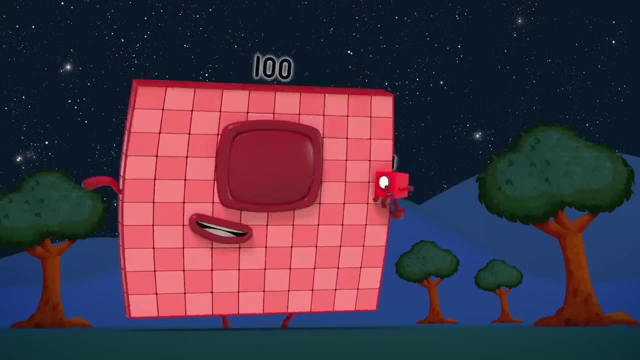 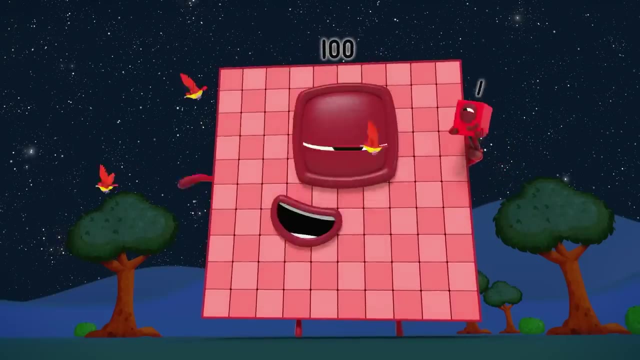 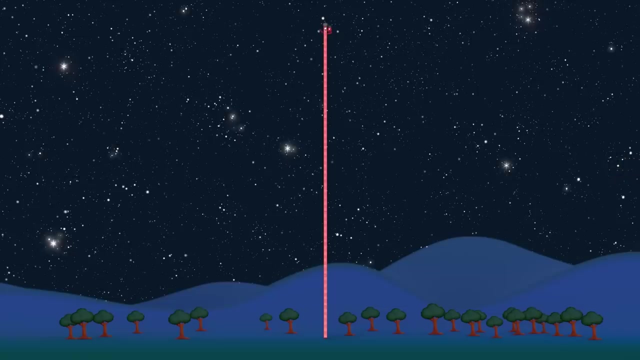 So big. I'm really, really, really big. I am gigantic Gigantic. Did I mention I was? I was big, Mm-hmm, I'm taller than the tallest tree. No one here's as tall as me Because I'm big. 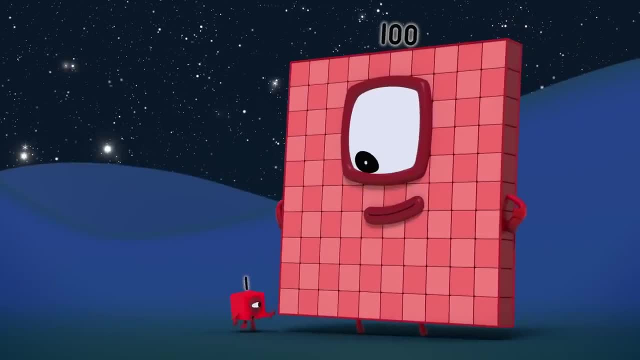 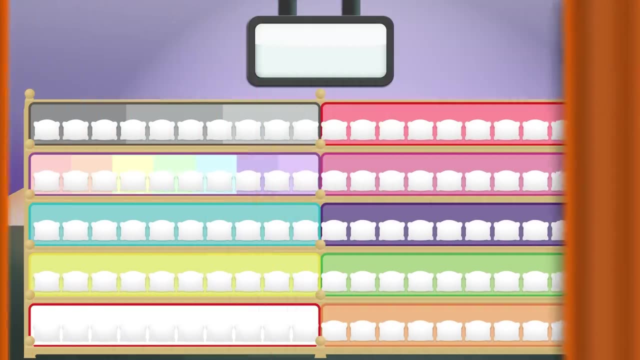 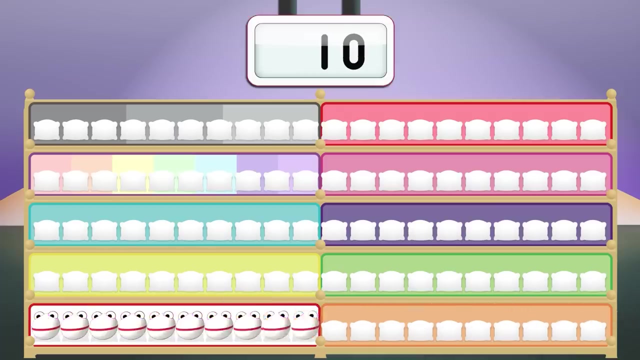 I'm really very big Look. One: two Number dogs- Ha-ha-ha, Ha-ha-ha. Number dogs. Number dogs. Number dogs. Two Number dogs Four. Four Number dogs. Six Number dogs Eight Number dogs: Ten. Ten Number dogs, Twelve Number dogs, Fourteen Number dogs. Sixteen, Eighteen, Eighteen, Twenty, Twenty, Twenty-two, Twenty-four, Twenty-six, Twenty, Twenty-eight, Twenty-eight, Thirty, Thirty, Thirty-two, Thirty-four. 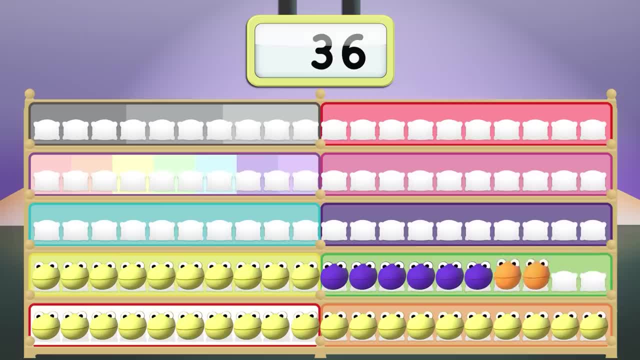 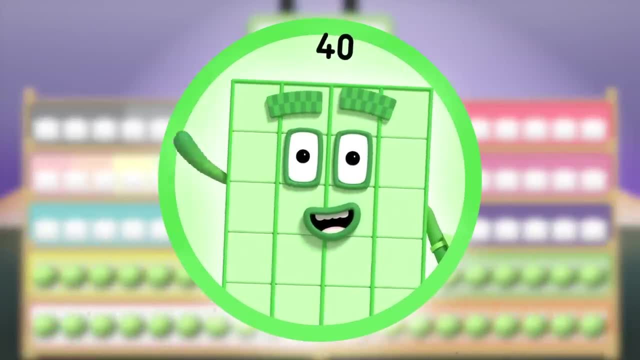 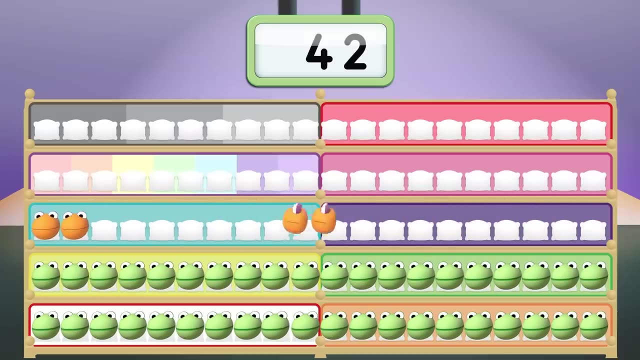 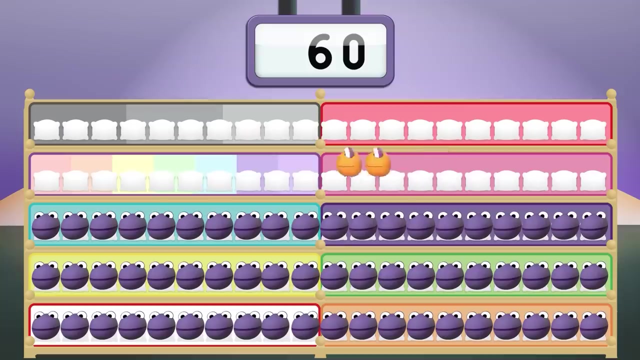 Thirty-six, Thirty-eight, Forty, Forty, Forty-two, Forty-four, Forty-six, Forty-eight, Fifty, Fifty, Fifty-two, Fifty-four, Fifty-six, Fifty-six, Fifty-eight, Sixty, Sixty, Sixty-two. 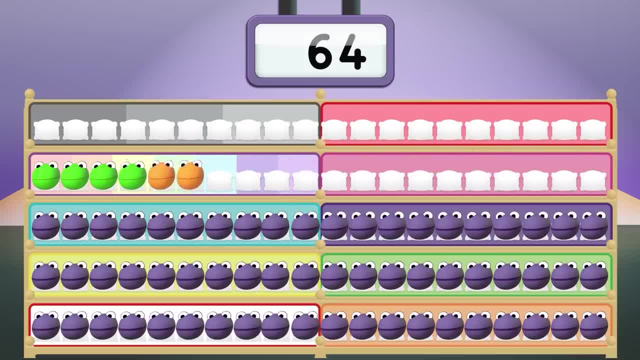 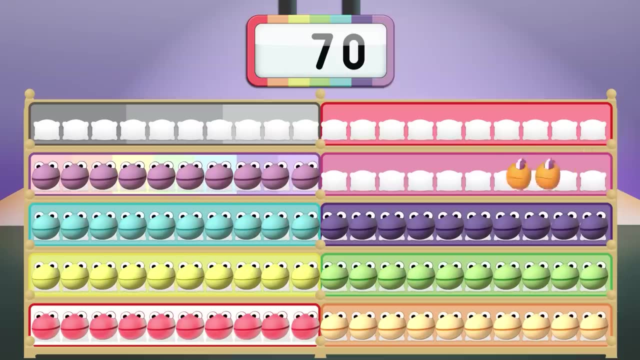 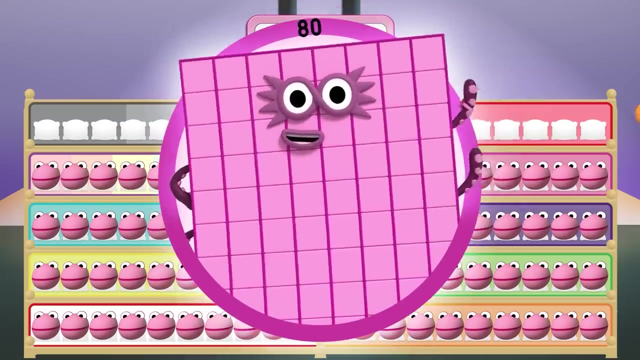 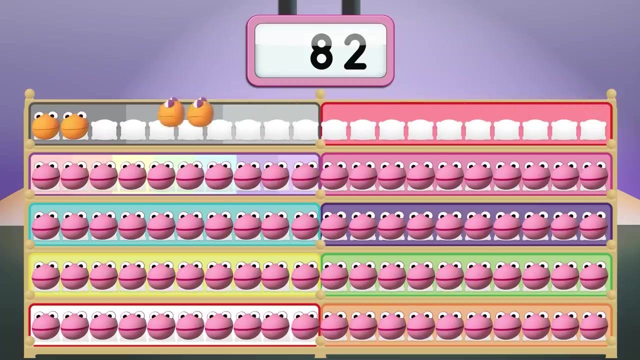 Sixty-four, Sixty-six, Sixty-six, Sixty-eight, Seventy, Seventy, Seventy-two, Seventy-four, Seventy-six, Seventy-eight, Eighty, Eighty, Eighty-two, Eighty-four. 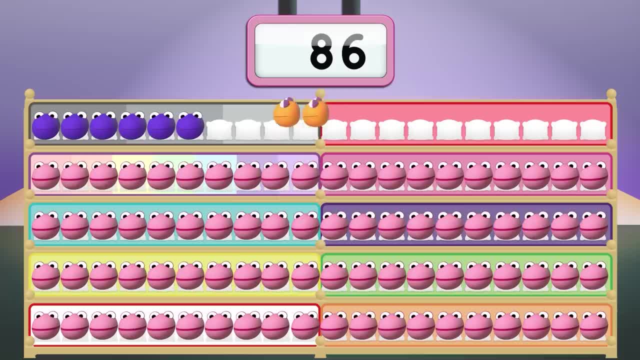 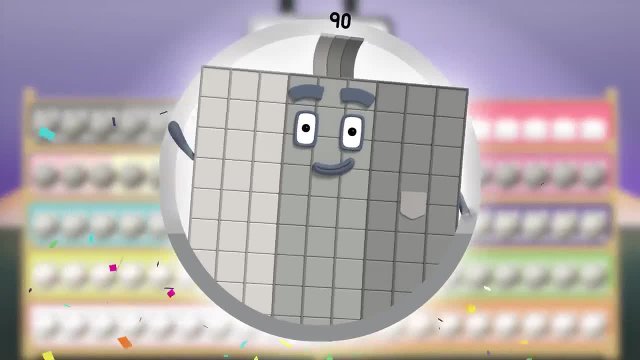 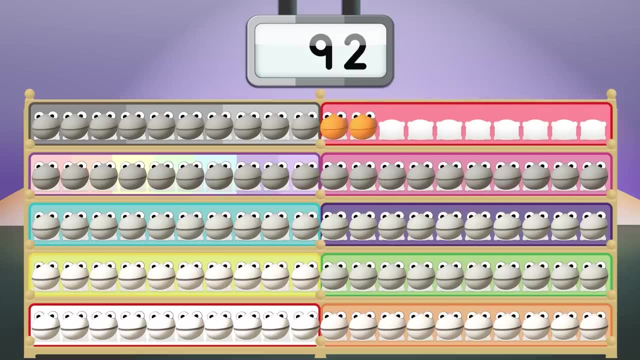 Eighty-six, Eighty-eight, Ninety, Ninety, Ninety-two, Ninety-nine, Ninety-two, Ninety-three, Ninety-six, Ninety-eight, Ninety- oleh elemental Ninety-four, Ninety-six. 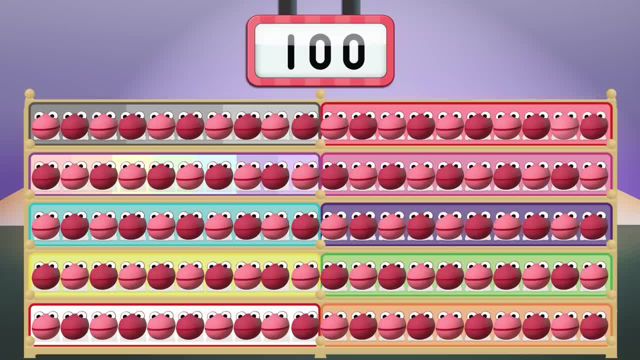 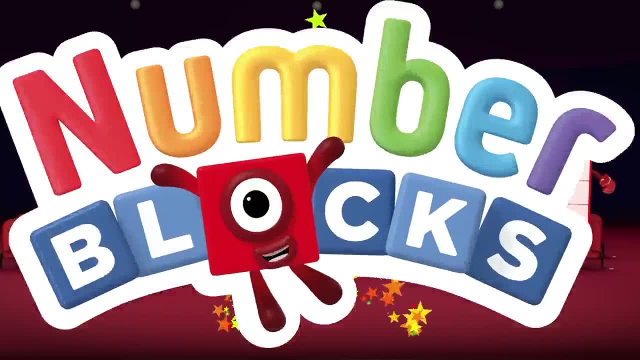 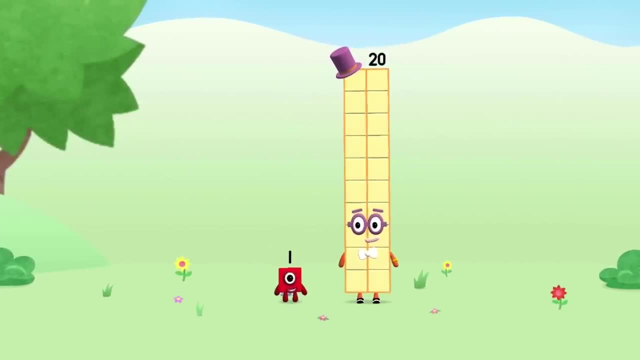 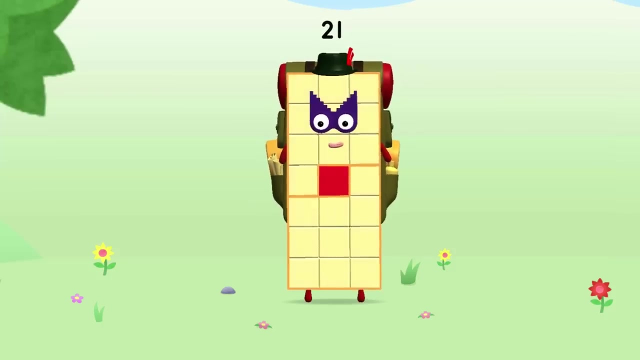 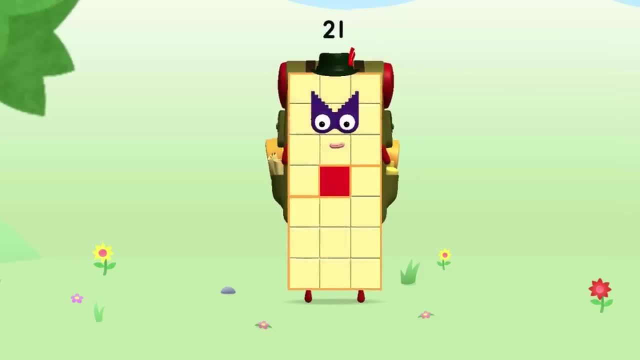 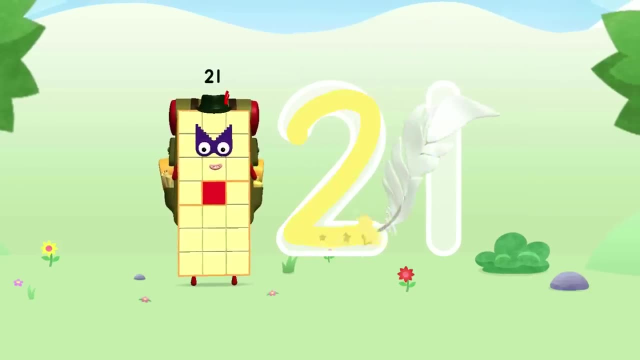 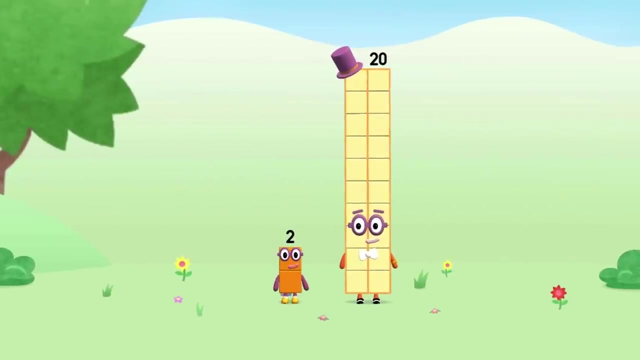 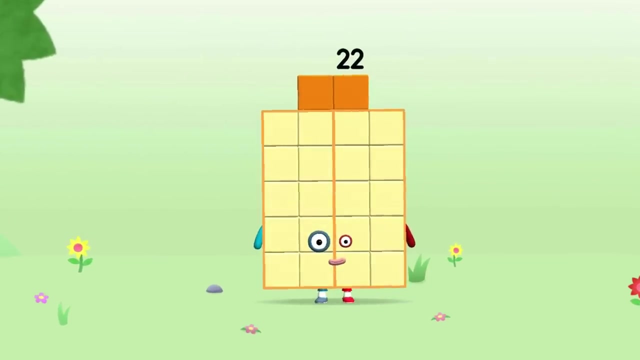 This number block is made up of twenty-one blocks. There's always more to explore. Yay, You're about to meet number block twenty-two. Can you add two to twenty and make number block twenty-one? Yay, This is number block twenty-two. 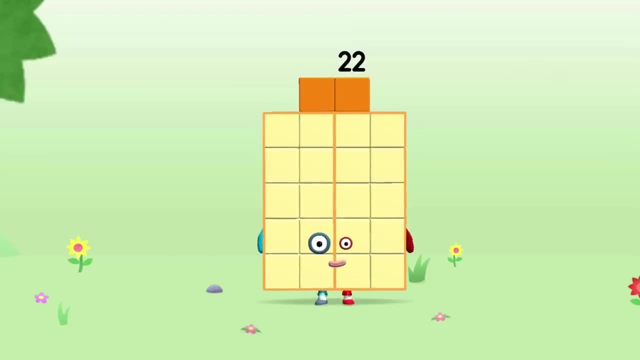 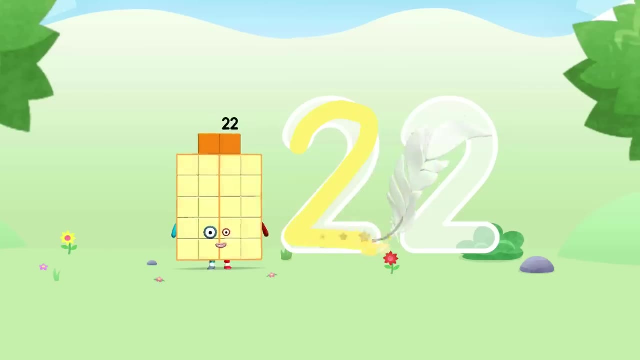 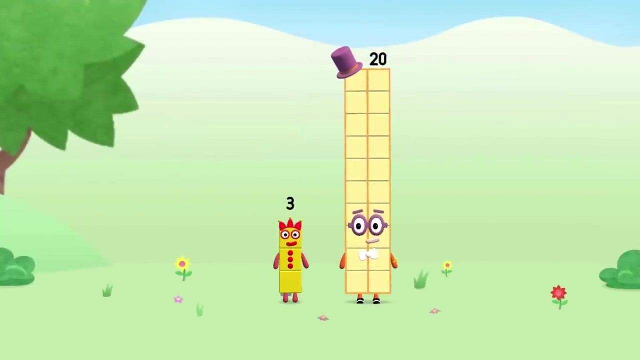 This number block is made up of twenty-two blocks And two football teams. Can you add one to twenty and make number block twenty-three? Brilliant, You're about to meet number block twenty-three. Can you add three to twenty and make number block twenty-three? 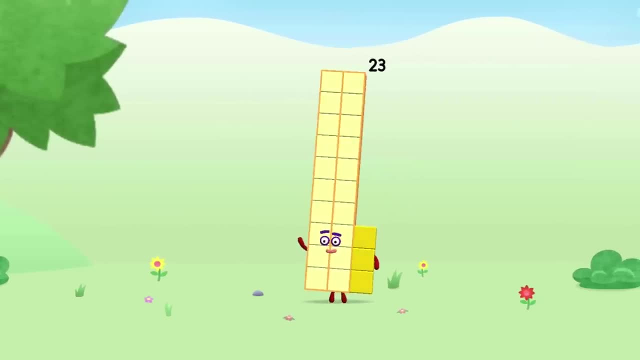 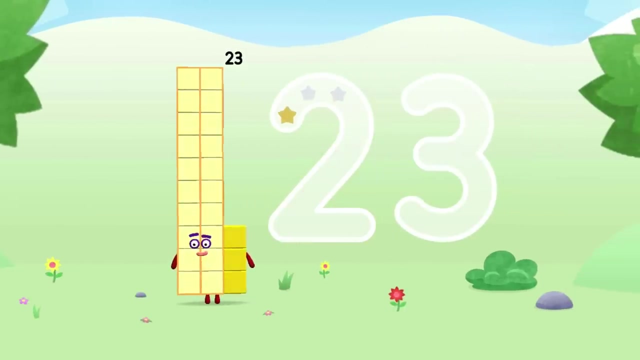 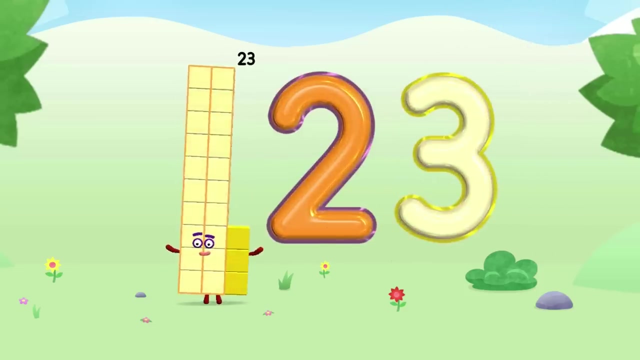 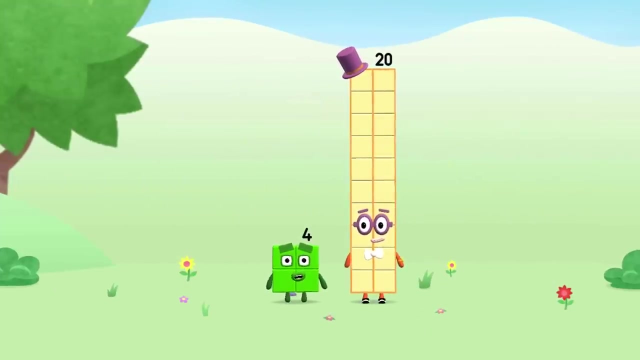 Drag number block three. Brilliant, This is number block twenty-three. This number block is made up of twenty-one blocks, Twenty-three blocks. Hooray, You're about to meet number block twenty-four. Can you add four to twenty and make number block twenty-four? 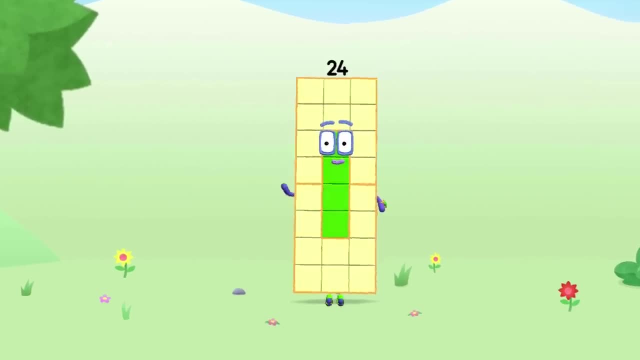 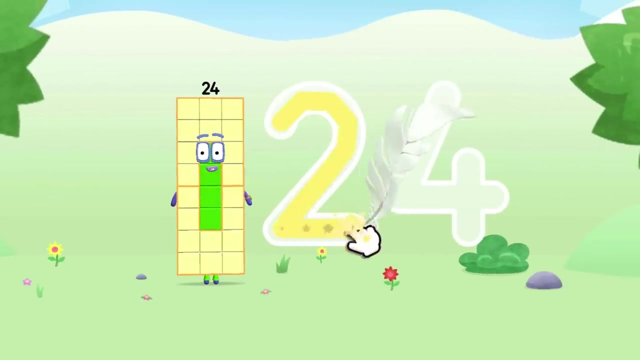 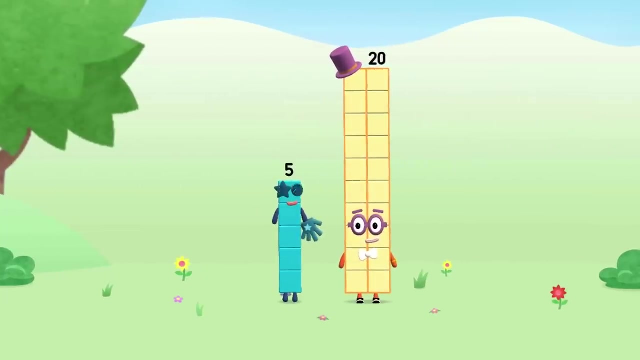 Drag number block four. Brilliant, This is number block twenty-four. This number block is made up of twenty-four blocks. I'm a super-duper rectangle. Brilliant, You're about to meet number block twenty-five. Can you add five to twenty and make number block twenty-five? 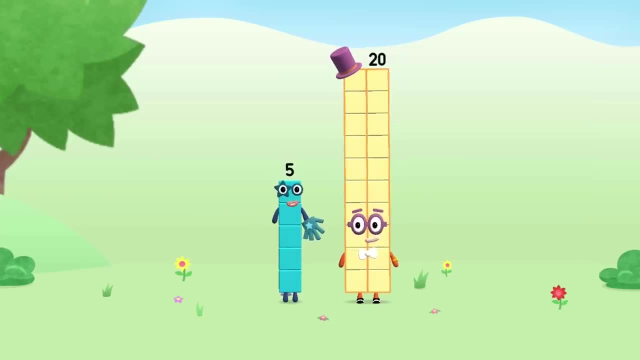 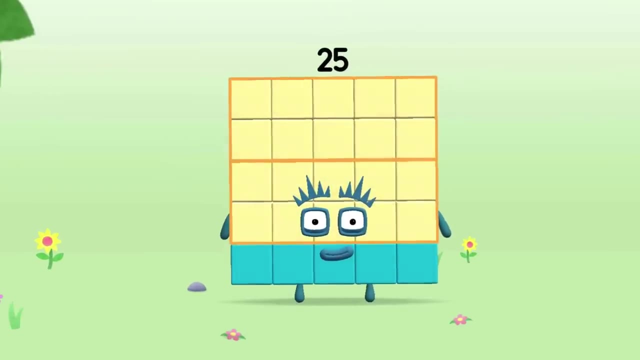 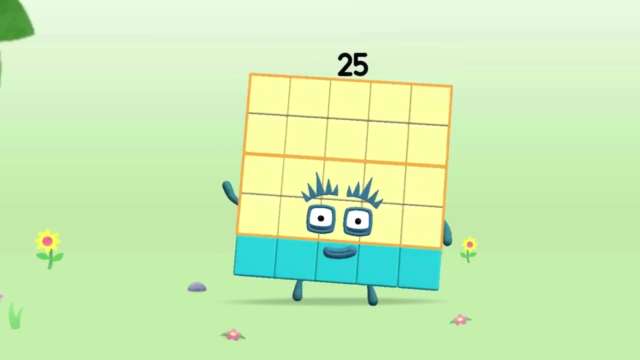 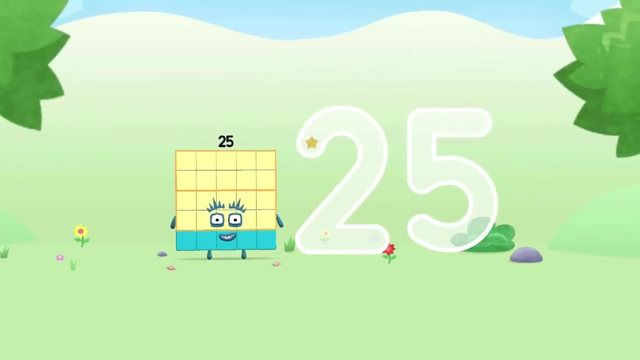 Drag number block five onto number block Yay. This is number block twenty-five. This number block is made up of twenty-five blocks. Five, lots of five. You're about to meet number block twenty-six. Use your finger to trace the number. 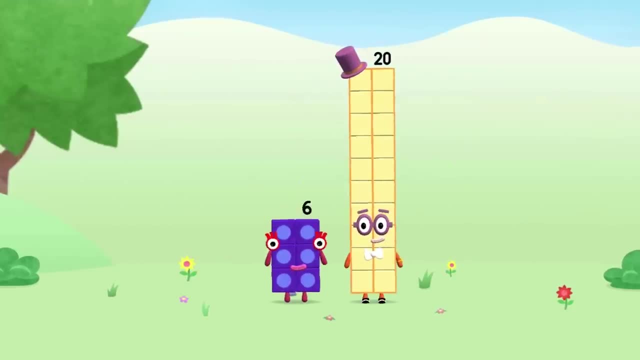 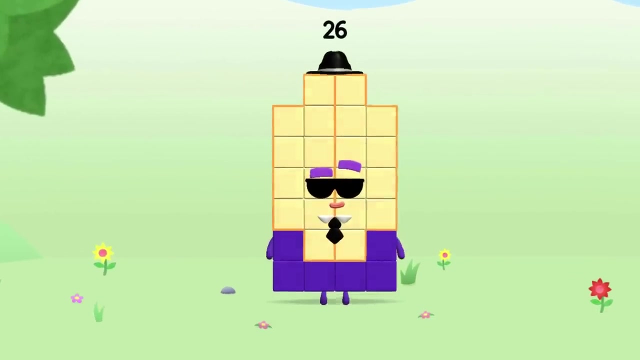 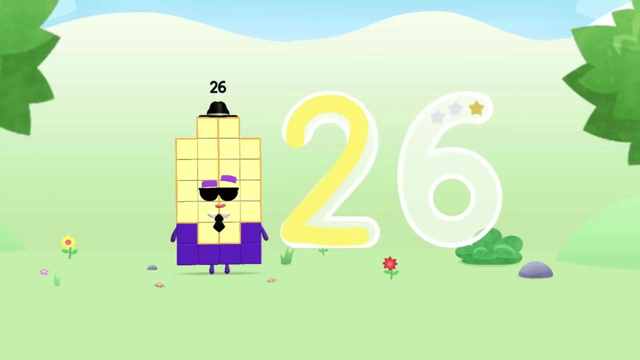 Well done. You're about to meet number block twenty-six. Can you add six to twenty and make number block Twenty-six Drag? Well done. This is number block twenty-six. This number block is made up of twenty-six blocks. Well done. 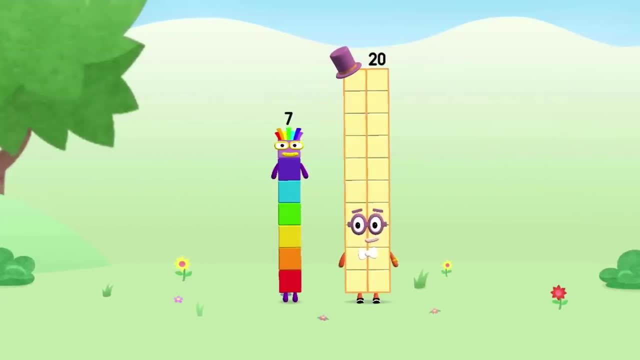 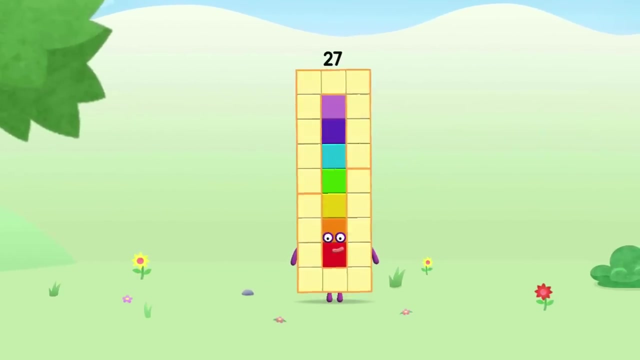 You're about to meet number block twenty-seven. Can you add seven to twenty and make number block twenty-seven? Drag number block Amazing. This is number block twenty-seven. This number block is made up of twenty-seven blocks. I'm a cube. 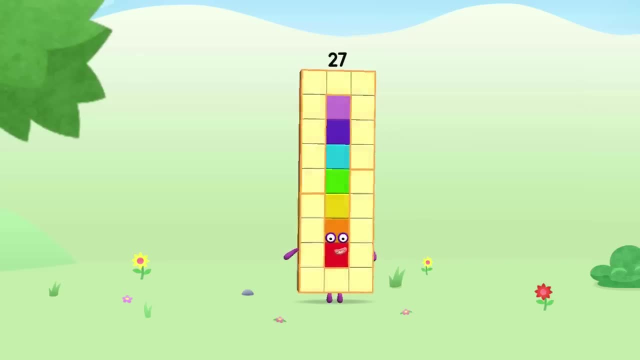 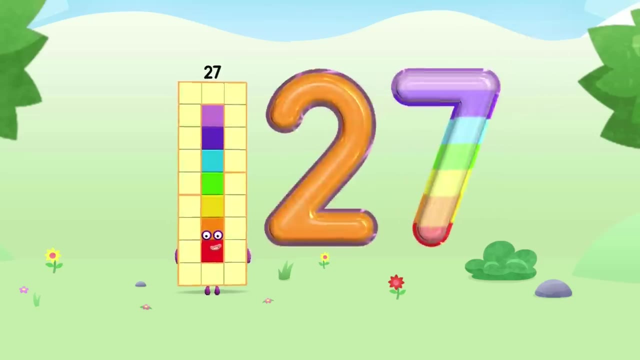 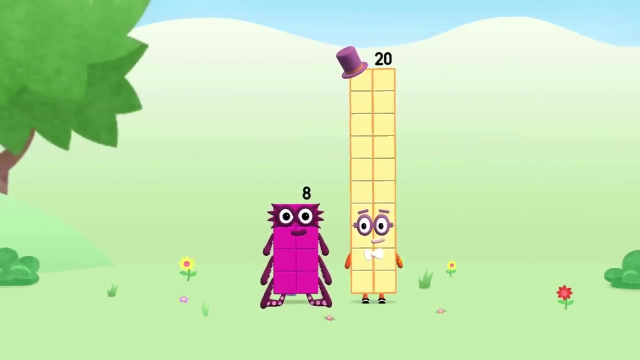 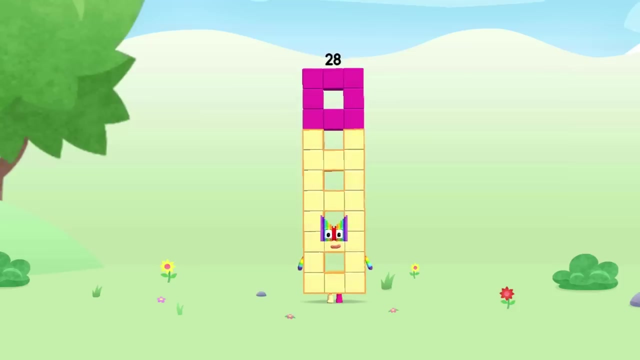 Three by three by three. Whee, Well done. You're about to meet number block twenty-eight. Can you add Eight to twenty and make number block twenty-eight? Amazing, This is number block twenty-eight. This number block is made up of twenty-eight blocks. 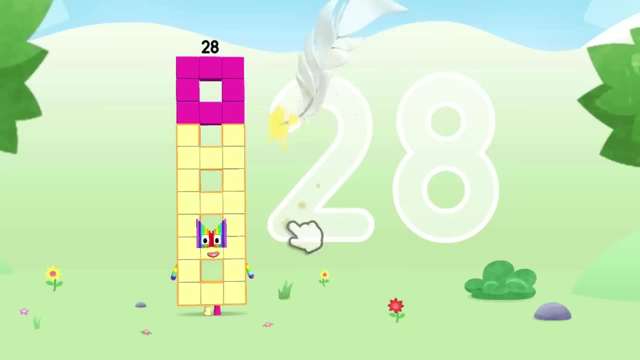 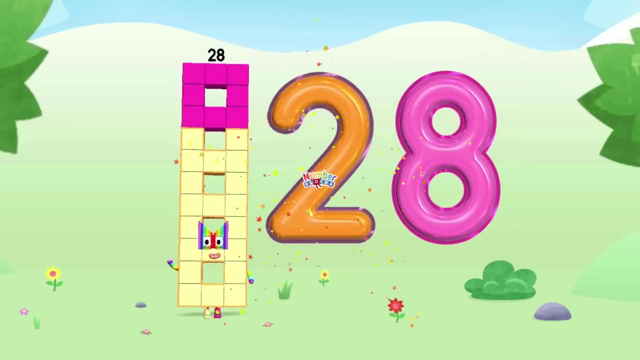 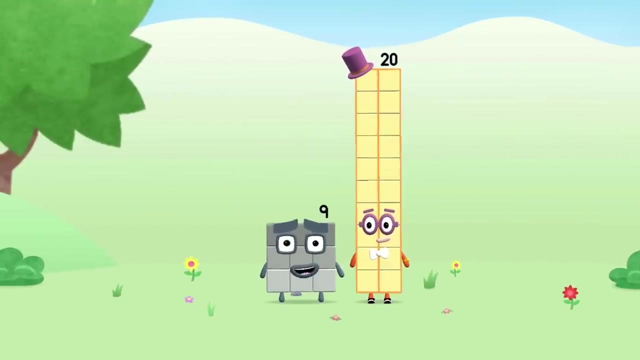 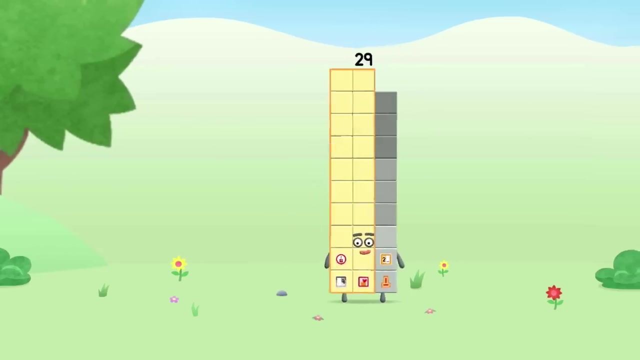 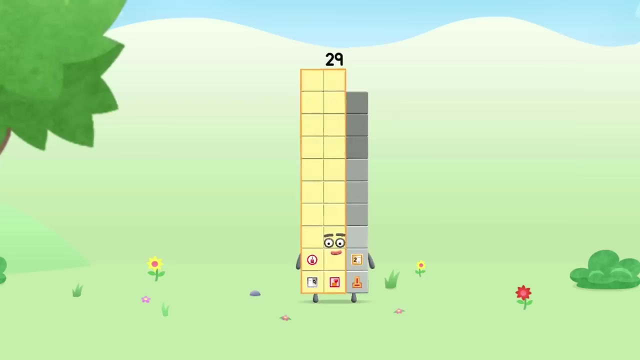 a pattern pioneer, try to keep your finger on the screen. well done, you're about to meet number block 29. can you add 9 to 20 and make number block 29 amazing? this is number block 29. this number block is made up of 29 blocks. 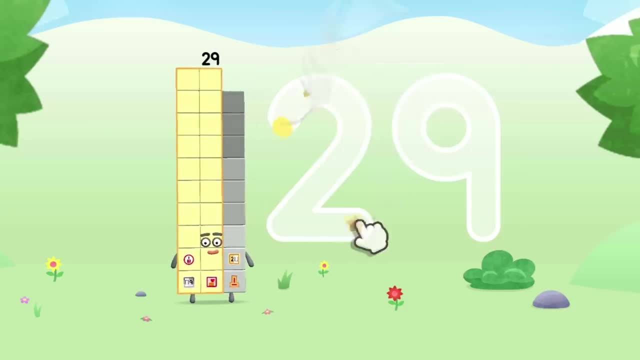 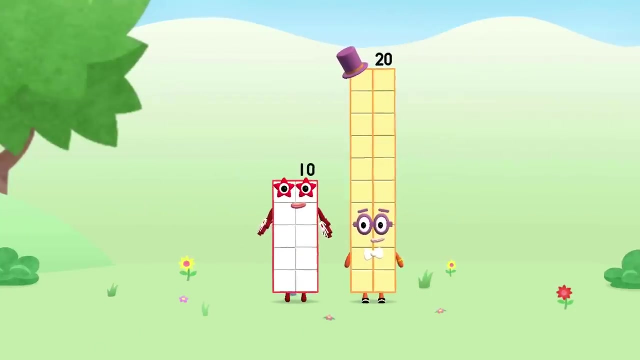 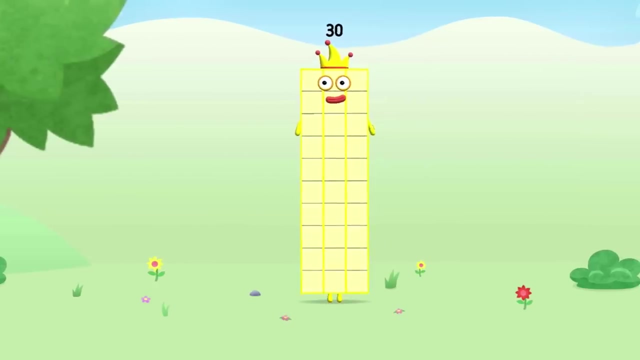 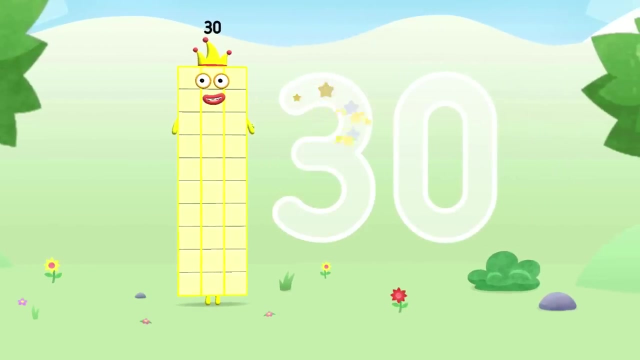 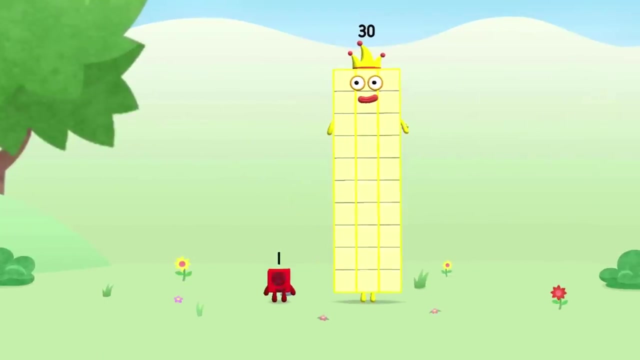 yay, you're about to meet number block 30. can you add 10 to 20 and make number block 30? this is number block 30. this number block is made up of 30 blocks. I am 30, the big entertainer. you're about to meet number block 31. can you add 1 to 30? well done, this is. 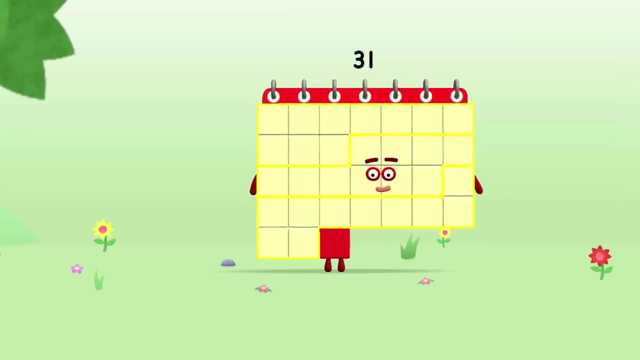 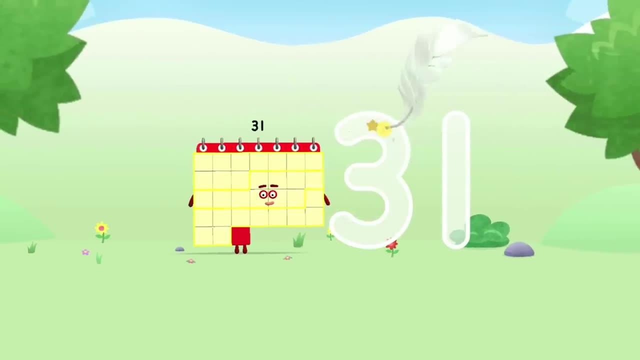 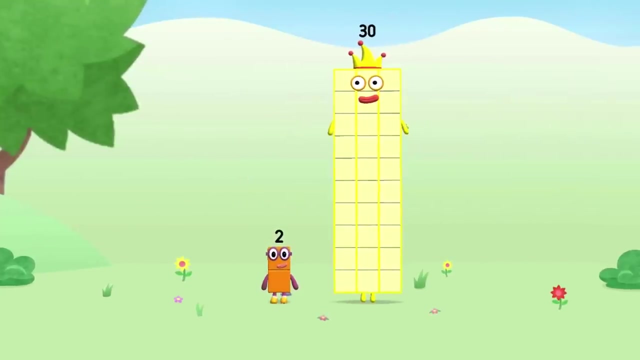 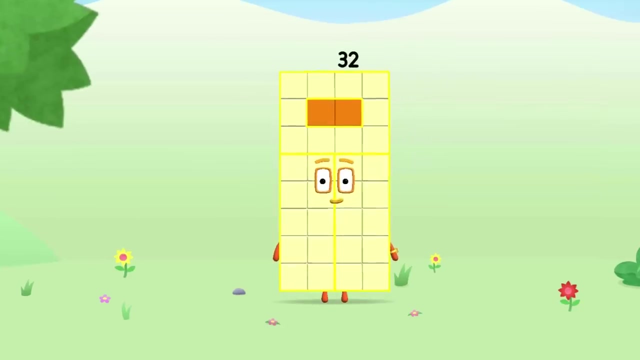 number block 31. this number block is made up of 31 blocks. amazing, you're about to meet number block 32. can you add 2 to 30 and make number block 32? drag number block 2. amazing, this is number block 32. this number block is made up of 32 blocks. 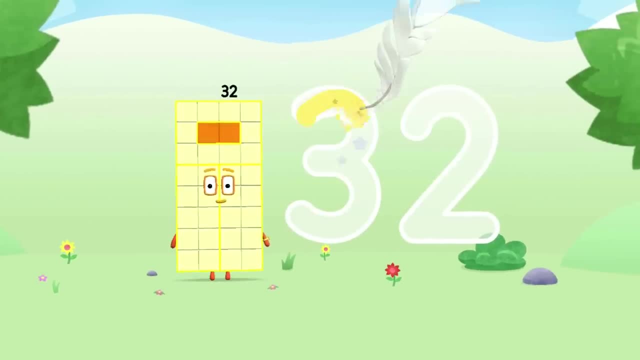 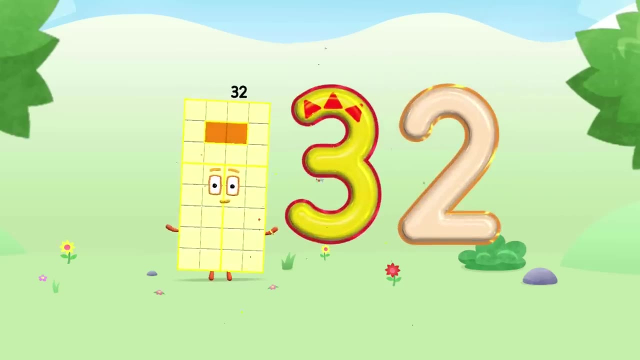 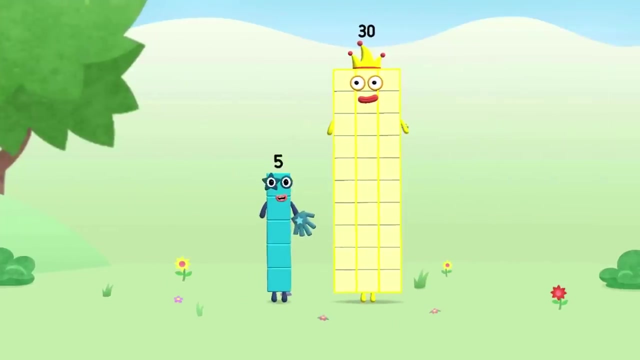 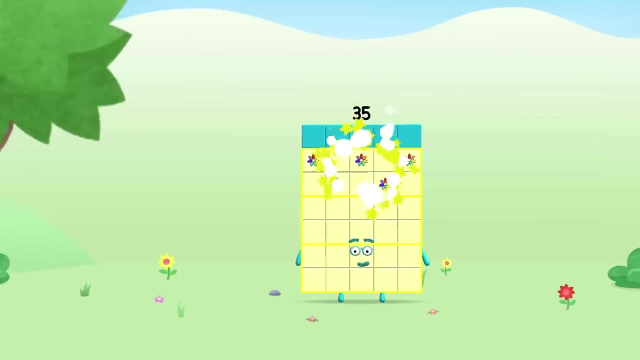 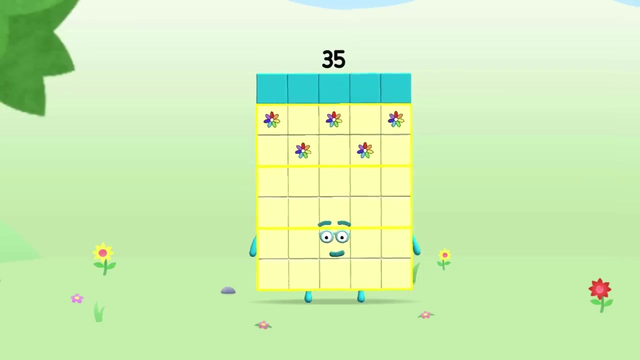 you're about to meet number block 35. can you add 5 to 30 and make number block 35? this is number block 31 is made up of 32 blocks. Sam's croc said the church is F, a big entertainer drag number. brilliant. this is number block 35. this number block is made up of. 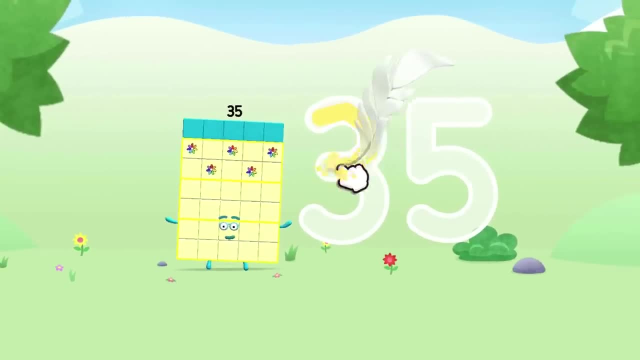 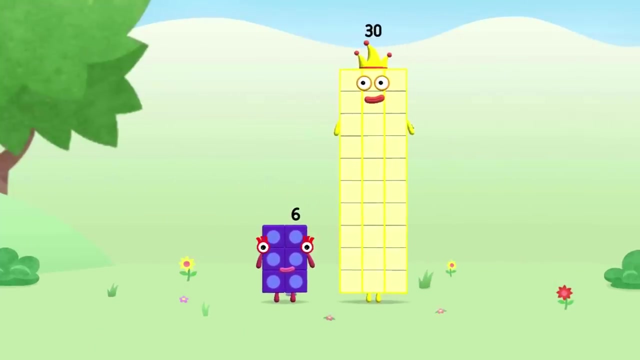 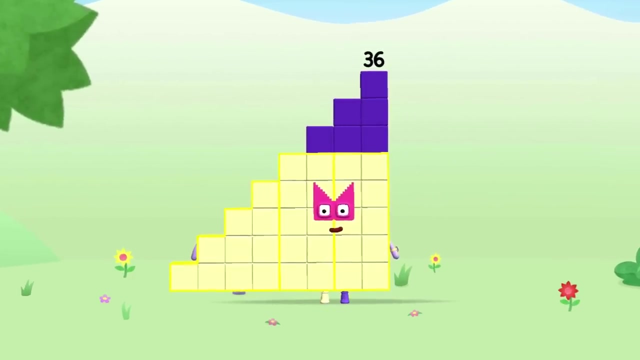 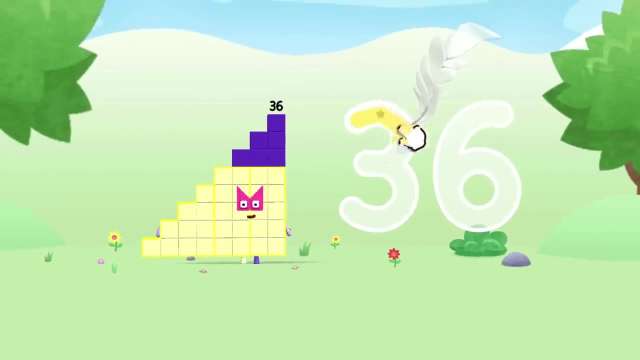 35 blocks. hooray, you're about to meet number block 36. can you add six to 30 and make number block 35 blocks 36.. Spot on, This is number block 36.. This number block is made up of 36 blocks. Try. 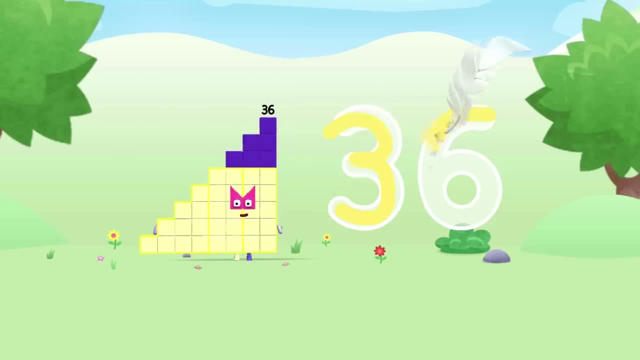 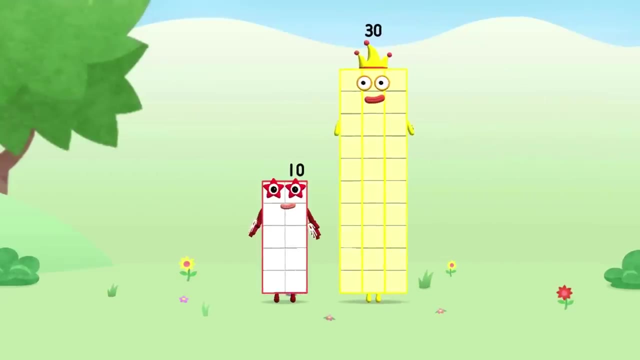 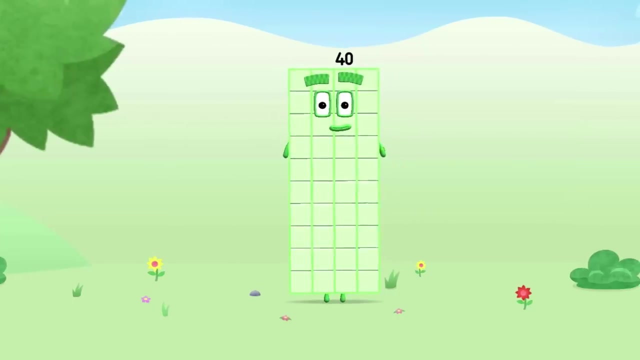 to keep your finger on the screen. Yay, You're about to meet number block 40.. Can you add 10 to 30 and make number block 40? Drag number block 10 onto number block. Amazing, This is number block 40. This number block is made up of 40 blocks. I love. 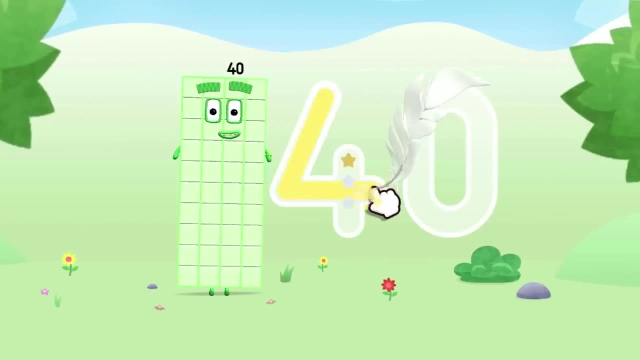 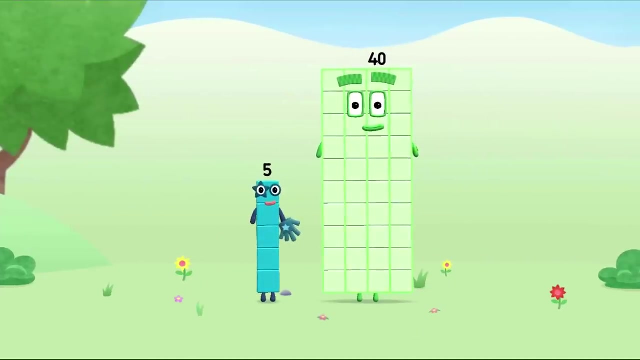 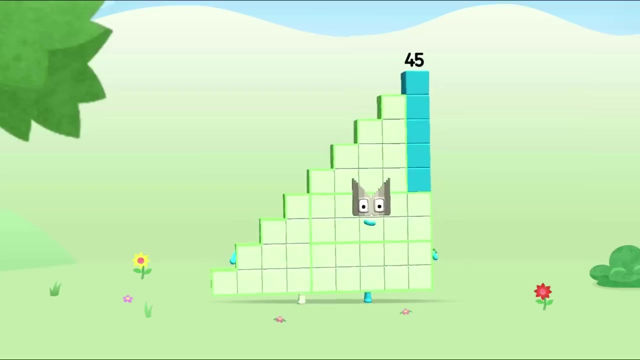 rectangles. Yay, You're about to meet number block 45.. Can you add 5 to 40 and make number block 45?? Drag number block 5 onto number block. Hooray, This is number block 45.. This number block is made up of 45 blocks. 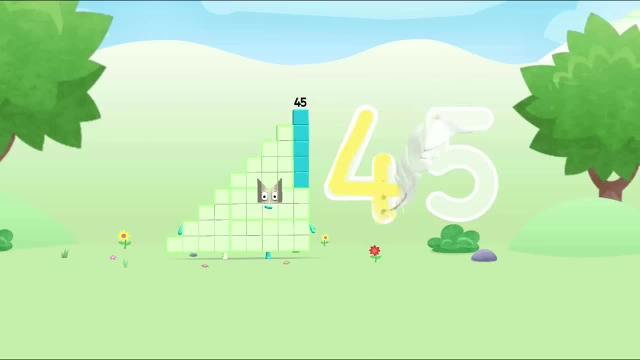 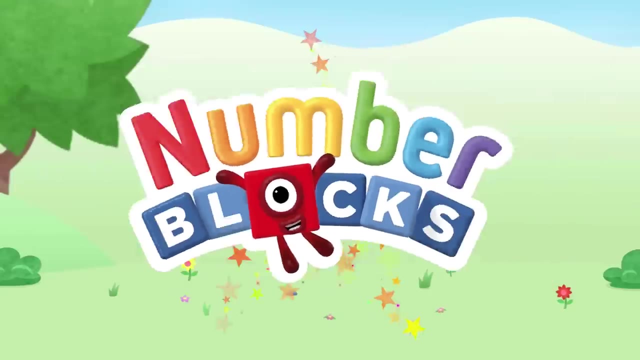 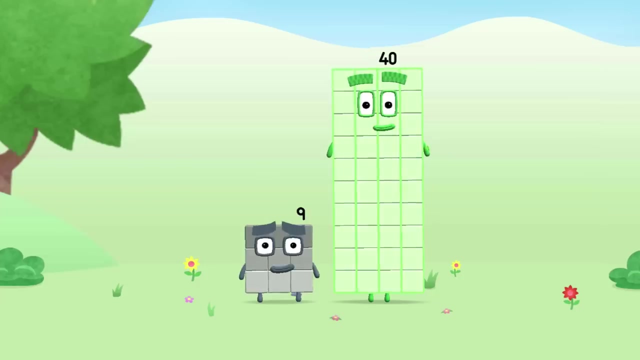 Try to keep your finger on the screen. Yay, You're about to meet number block 49.. Can you add 9 to 40 and make number block 49?? Drag number block 9 onto number block. Hooray, Amazing, This is number block 40.. This number block is made up of 40 blocks. Can you add? 9 to 40 and make number block 49? Drag number block 9 onto number block. Hooray, This is number block 49.. This number block is made up of 47 blocks. Grrr, Woohoo, Amazing, You're about. 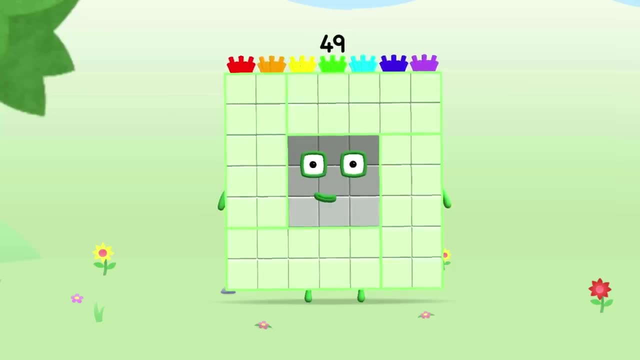 to meet number block 49.. Can you add 10 to 30 and make number block 45?. Drag number block 9 to 40 and make number block 49.. This number block is made up of 40 blocks. Well done You're. 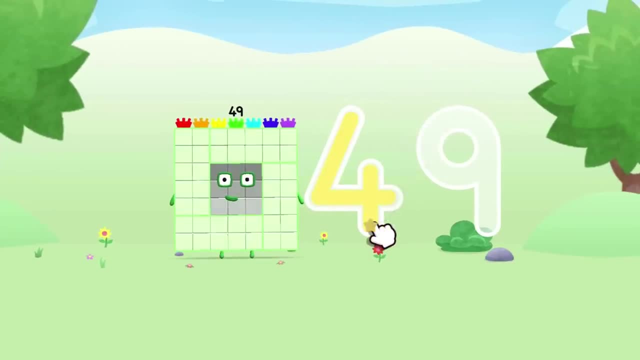 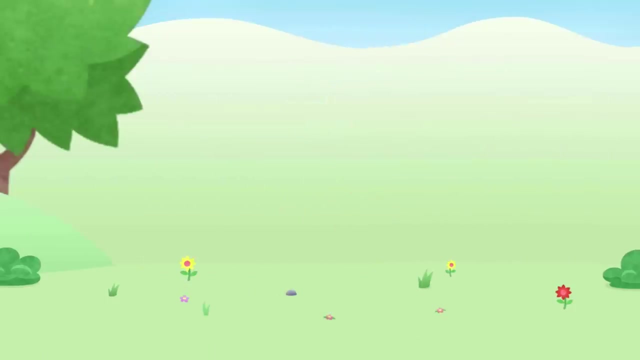 about to meet number block 59.. Can you add 2 to 60 and make number block 40?? hats off, Try to keep your finger on the screen. Yay, You're about to meet number block 59.. Can Can you add 10 to 40 and make number block 50?? 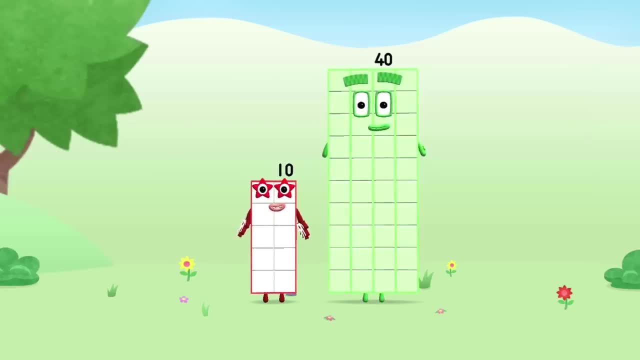 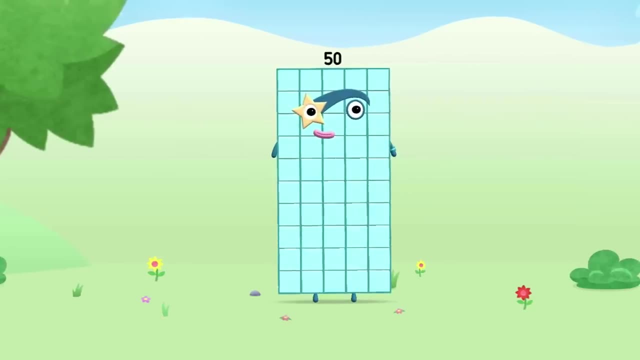 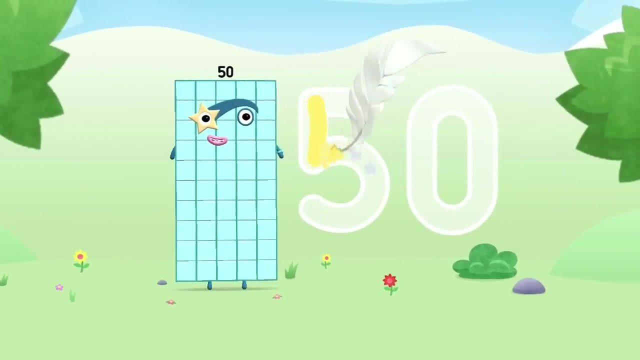 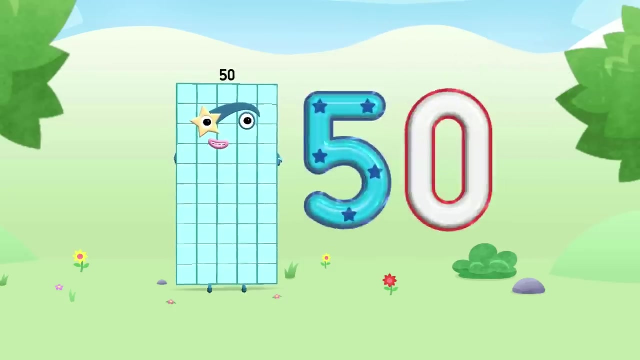 Drag number block 10 onto number block. Amazing, This is number block 50.. This number block is made up of 50 blocks. High fives all round. Give me ten fives. Yey, You're about to meet number block 55.. 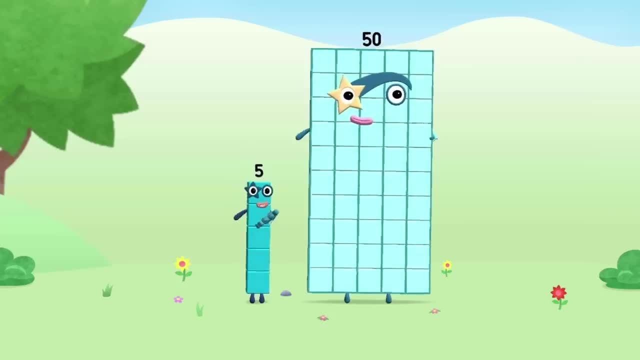 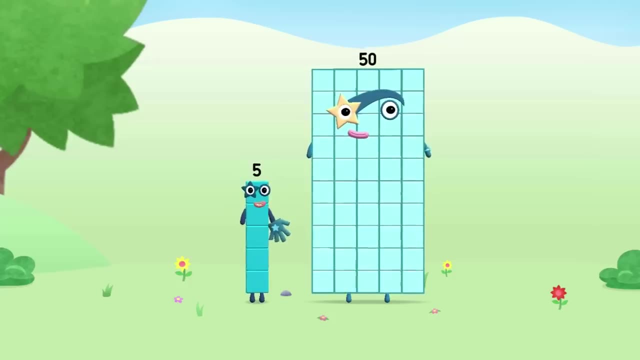 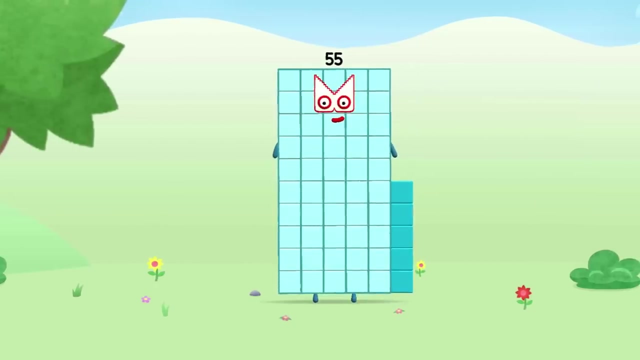 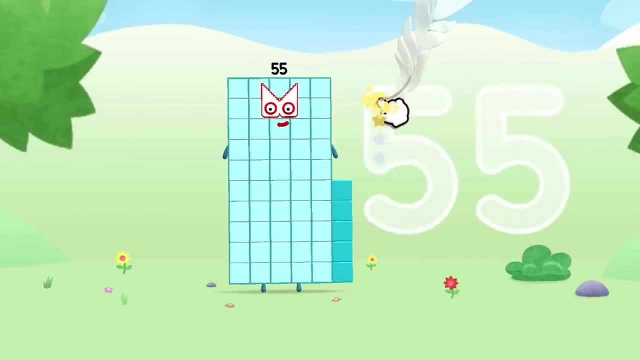 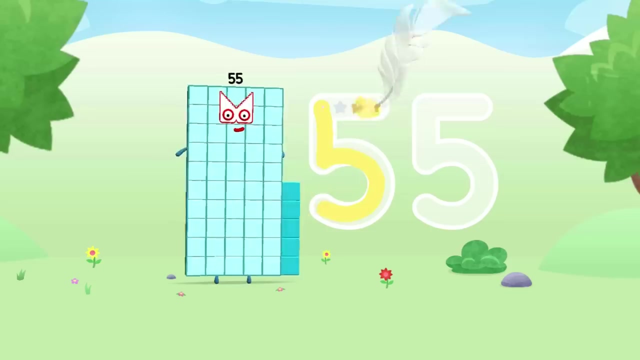 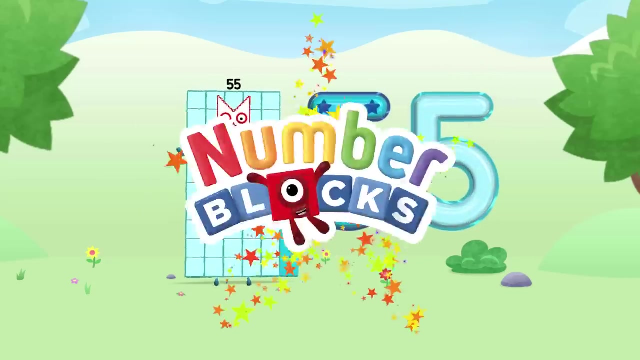 Can you add 5 to 50 and make number block 55?? Drag number block 5 onto number block. Amazing, This is number block 55.. This number block is made up of 55 blocks. Brilliant, You're about to meet number block 55.. 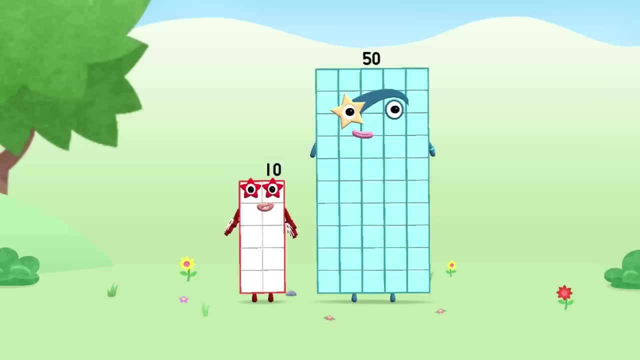 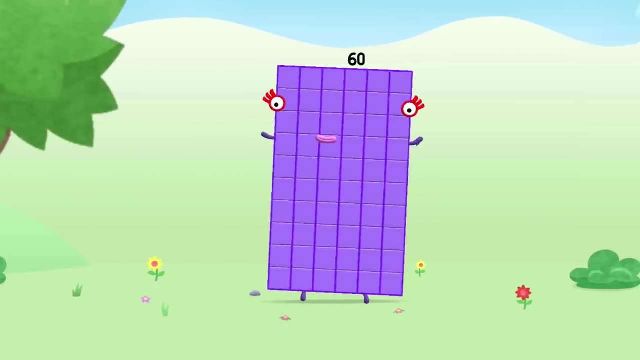 Can you add 10 to 50 and make number block 55?. You're about to meet number block 55. Drag number block 55.. Spot on, This is number block 60. This number block is made up of 60 blocks. 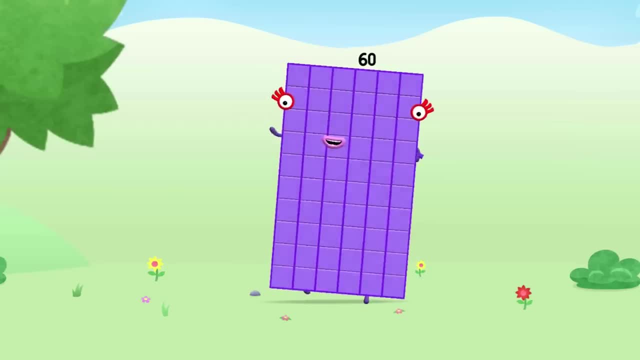 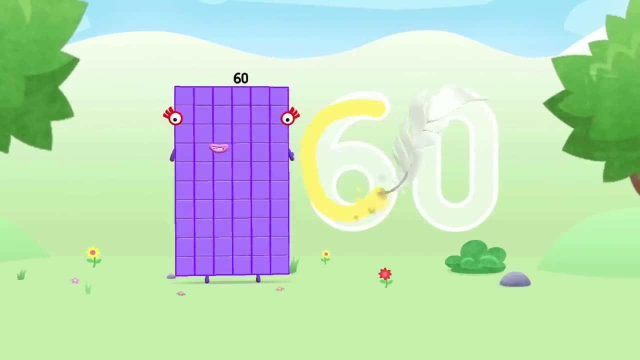 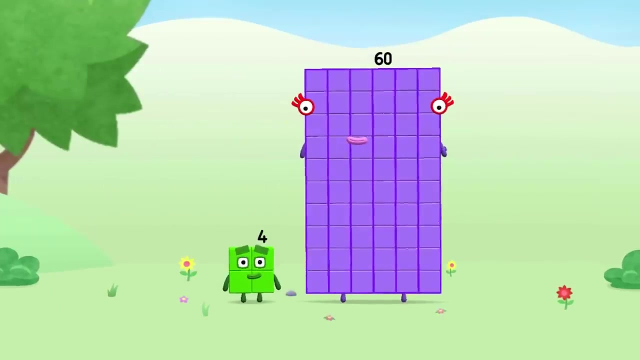 I am 60 here to play with 60 spots. Hip, hip, hooray- Try to keep your finger on the screen. Yay, You're about to meet number block 64. Can you add 4 to 60 and make number block 64? 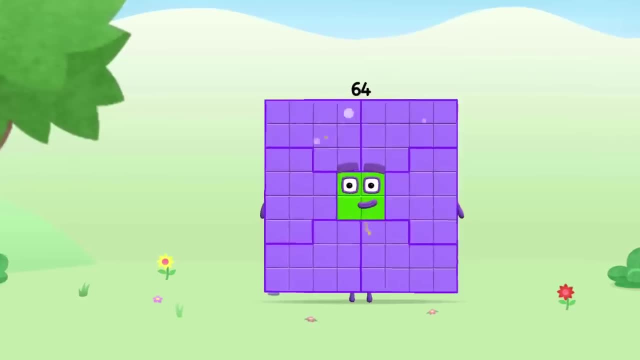 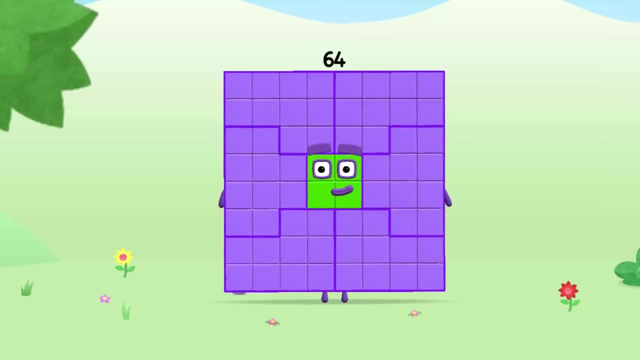 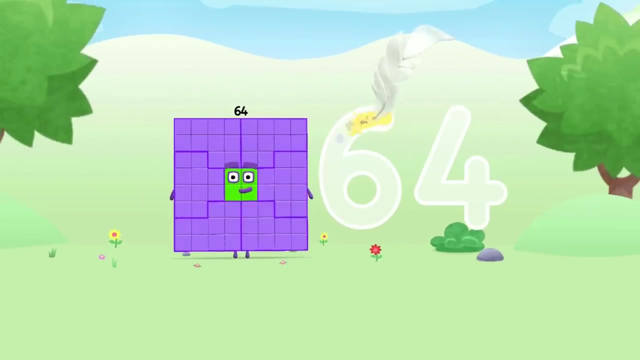 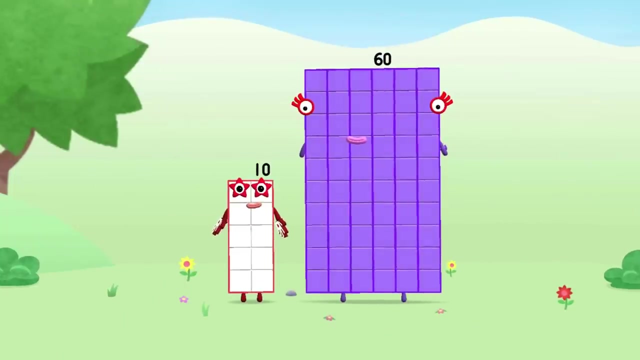 Drag number block 4: Spot on. This is number block 64. This number block is made up of 64 blocks Hooray. You're about to meet number block 70. Can you add 10 Hooray To 60 And make number block 70? 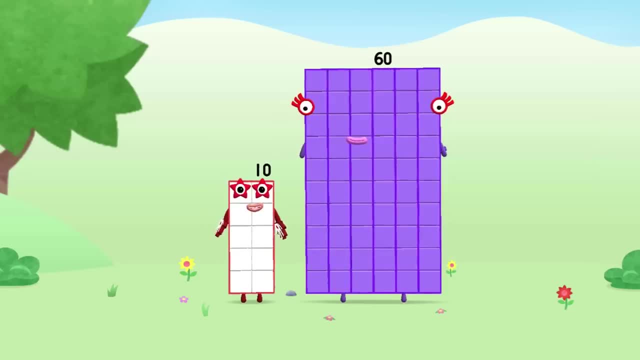 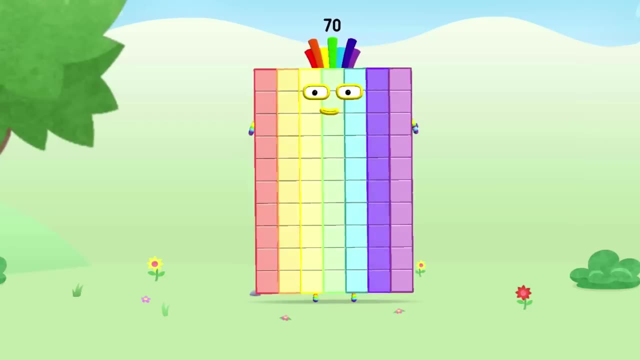 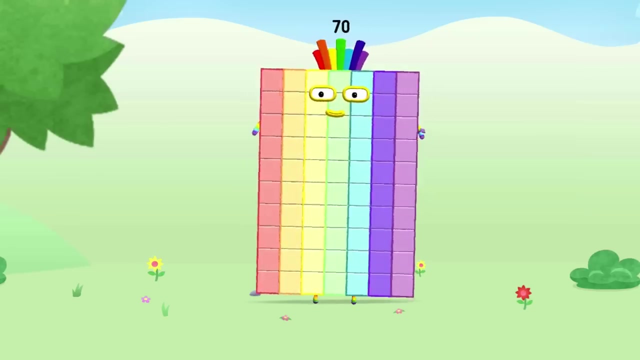 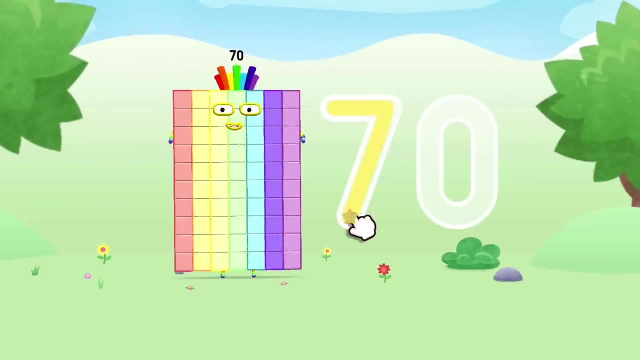 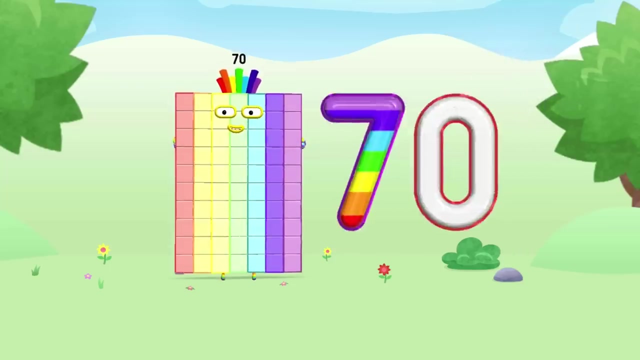 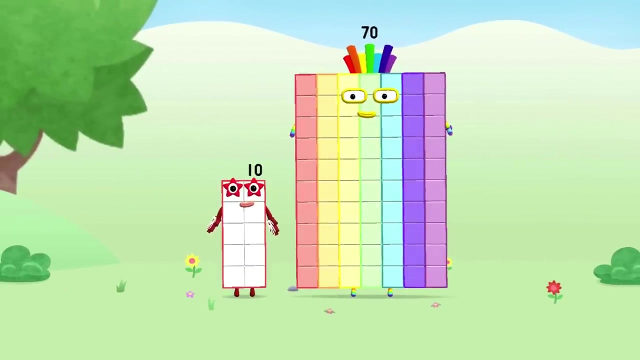 Drag number block 10 Onto number block Spot on. This is number block 70. This number block is made up of 70 blocks. As luck would have it, I'm 7 tens Spot on. You're about to meet number block 80. 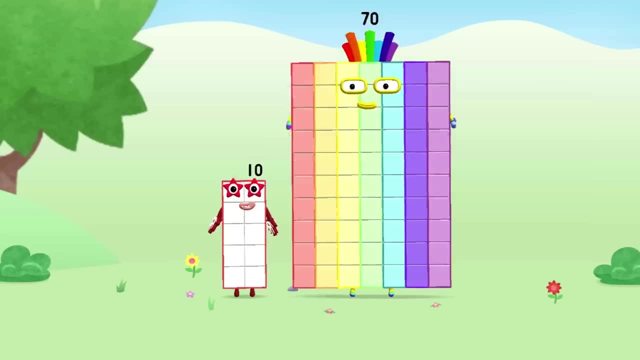 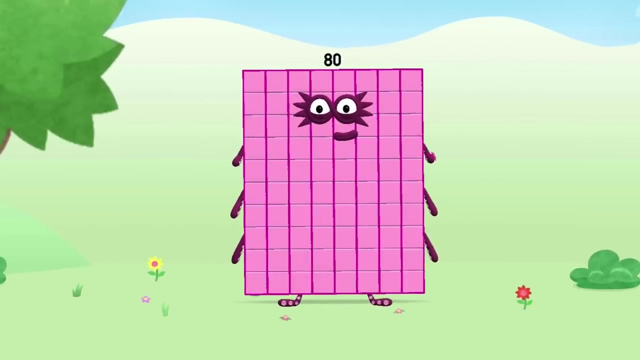 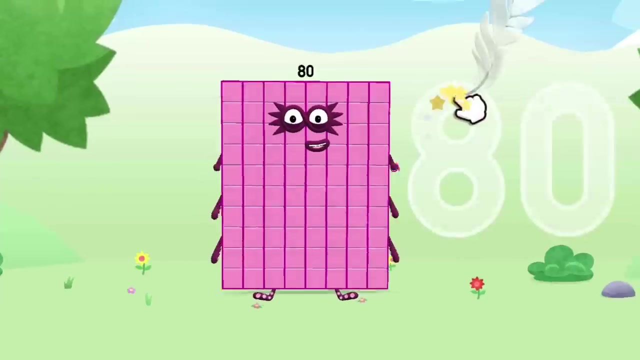 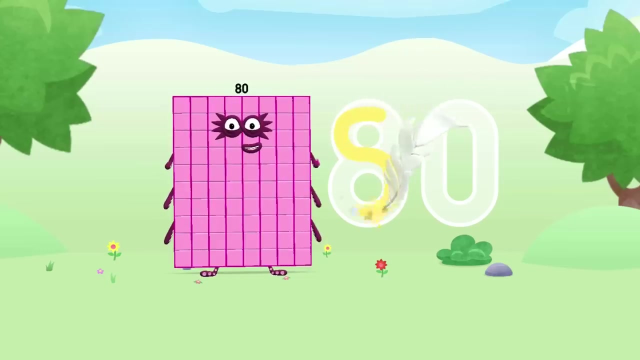 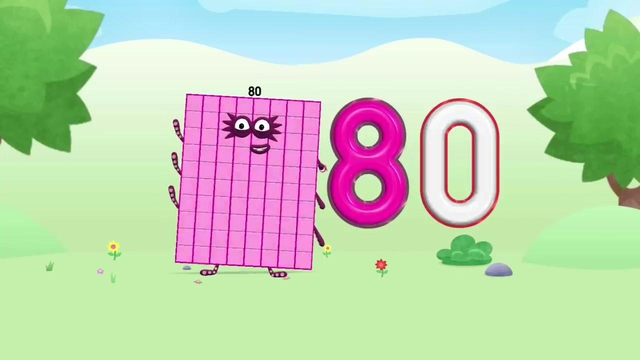 Can you add 10 To 70 And make number block 80? Drag number block 10. Hooray, This is number block 80. This number block is made up of 80 blocks. Dinocto block smash Spot on. You're about to meet number block 81.